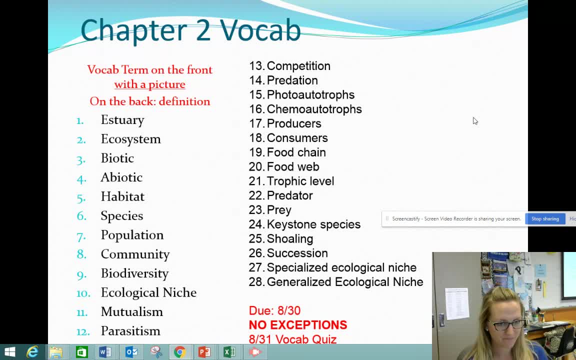 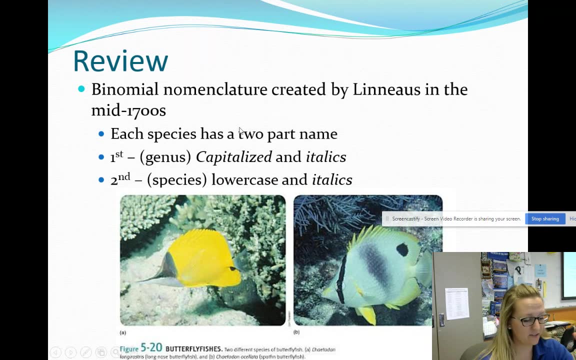 shoaling succession. specialized ecological niche. generalized ecological niche. Okay, just a little bio review. So the way we name species is by their genus and then their species name. The genus is always going to be capitalized And it's in italics. The species name is lowercase and in italics At the bottom. 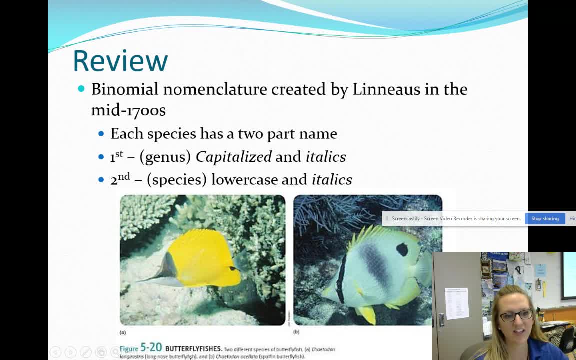 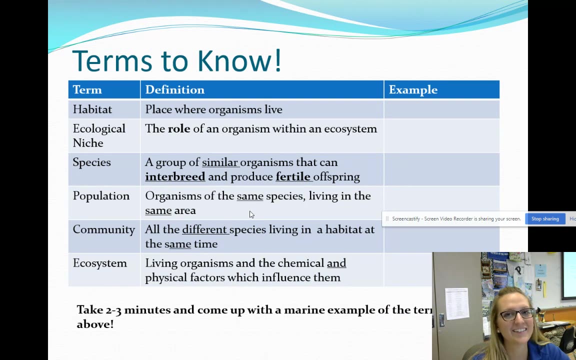 these are two different species of butterfly fish And you can see how they've written their name all the way at the bottom there. Okay, we're Homo sapiens, my favorite animals. Orchinus orca Carcharodon carcheris is the great white shark. Megoptera novanglidae is our humpback whale. 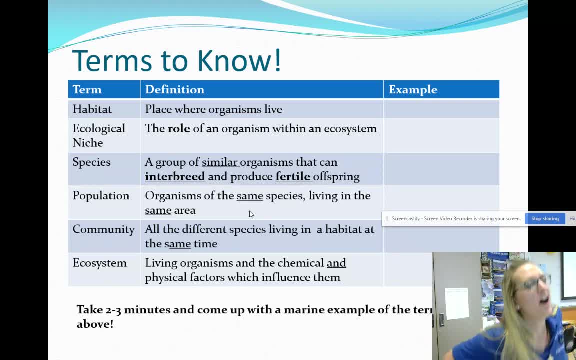 the big winged New Englander. Okay again, biodefinitions: Habitat is the place an organism lives. Ecological niche is one of those we have to be 150% on and be perfect with it. It is the role an organism plays in an ecosystem. The role 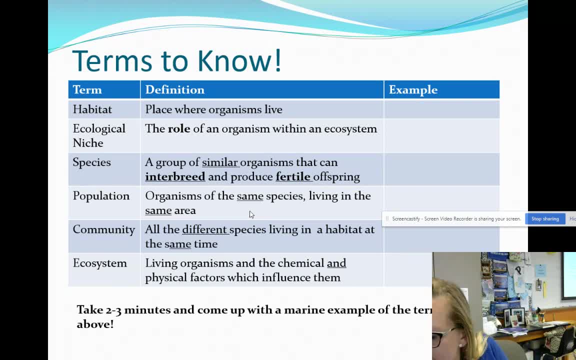 has to be the role. Okay, species, It's a group of similar organisms that can interbreed and produce fertile offspring. Sometimes species is a two-mark question, because they want to be a part of the ecosystem. So species is a group of similar organisms that can. 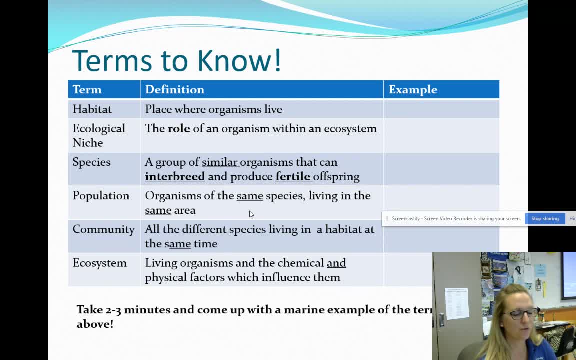 interbreed and produce fertile offspring. Sometimes species is a two-mark question because they want you to get that and produce fertile offspring. So you know we can have the tiger and the lion interbreed. They are similar species, They can interbreed and they produce a liger, but that 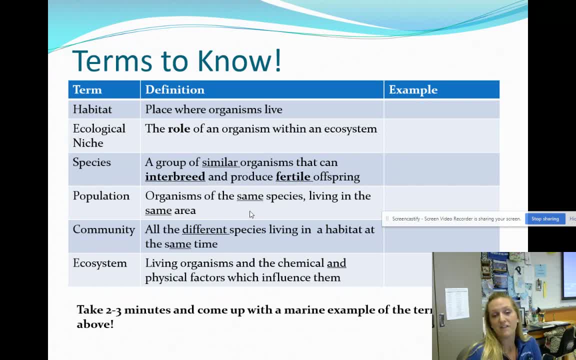 liger is sterile, So that baby liger, it's not fertile, It can't have more of its own. A liger can't mate with another liger and make more ligers. That can't happen. So they are not species. They 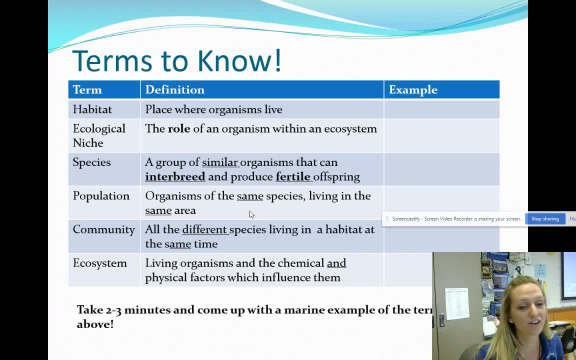 are hybrids. I'm going to call them a mutant. They're hybrids. A population is a group of the same species, So one species, and then a population is a group of the same species, So human population. We're all the same Community. Now we're adding in: 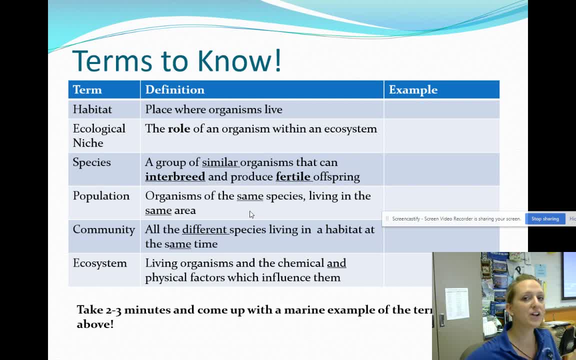 different populations together. So now you're not the same. So a community for us would be like students in the classroom plus the plants I have in the back. So that's. you know, they're living, but they are not our species. We could also include the plants in the back, So that's. 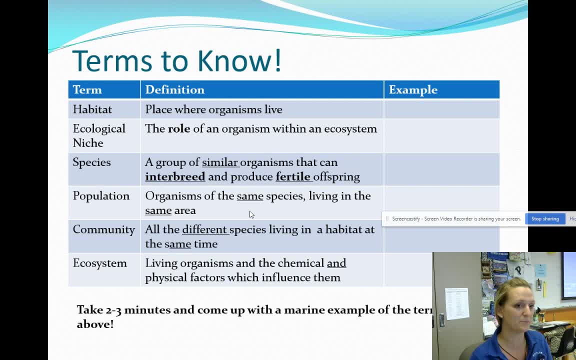 the bacteria that are all over the place. They're living, but they're not our species. That's a community: Communities. when they talk about community, it's all of the biotic, All of the living components in an ecosystem, is what the community is, Everything that's living Population. 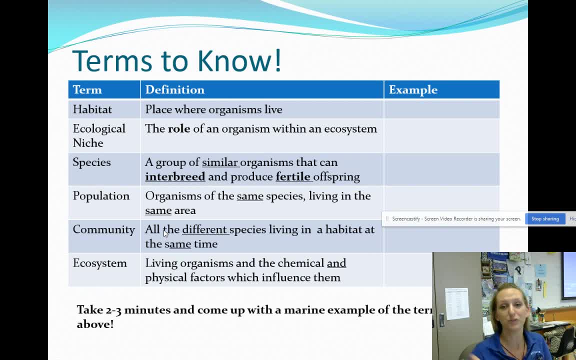 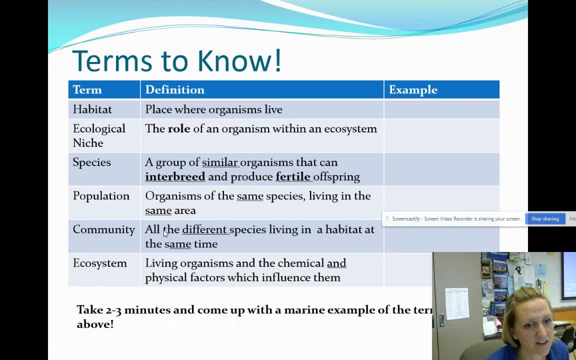 the same. You're not the same, You're not the same. So living organisms and the chemical and physical factors that influence them. So we have the living portion. I wonder, Just trying something out, Let's see Laser pointer. I'm sorry, Okay, Yeah, Living portions and the physical and chemical. 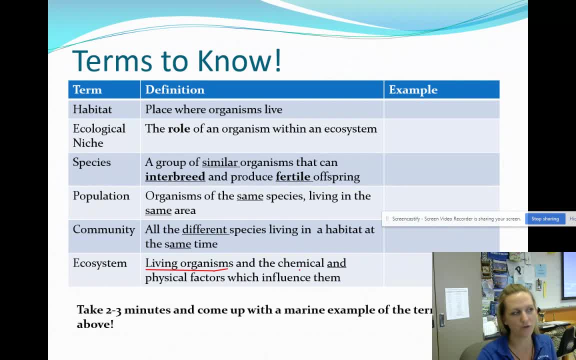 factors that influence them. So this is living and non-living. So, okay, What's the? what's the weather, like You know? is it raining right now? Is it cold? Is there? is it rocky? What's the soil like? Is it made of clay, Is it made of sand? Is it cloudy? So it would not be, obviously. 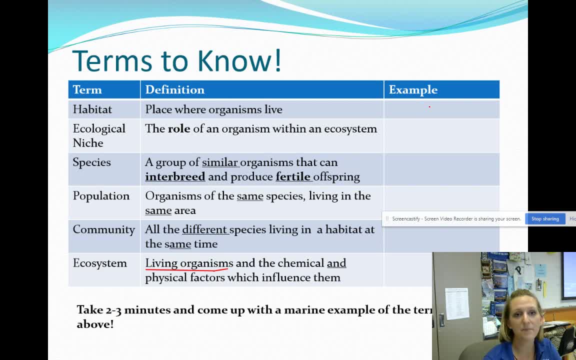 I'm not checking to make you see if you come up with your own examples. This would be a good thing for you to maybe do with your vocab right now, But it's not a bad idea for you to try this out. So my favorite thing, my favorite- is an orca, So their habitat is going to be like in the air, So 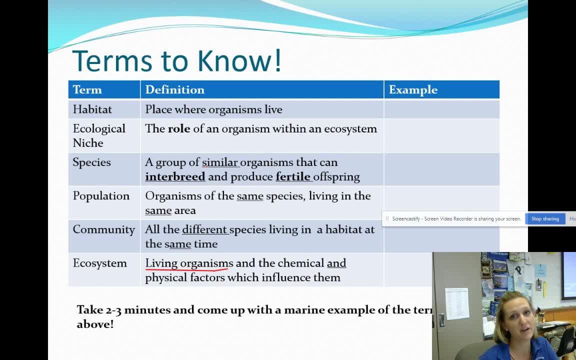 like in the Arctic, Their niche. they're an apex predator. The species would be one, orca, Orchinus. orca Population would be a pod of orcas. The community would be orcas living with seals and penguins and seabirds. That works, And then their ecosystem would be in the Arctic Ocean, The 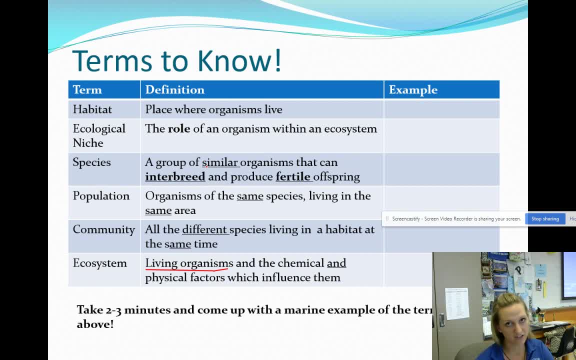 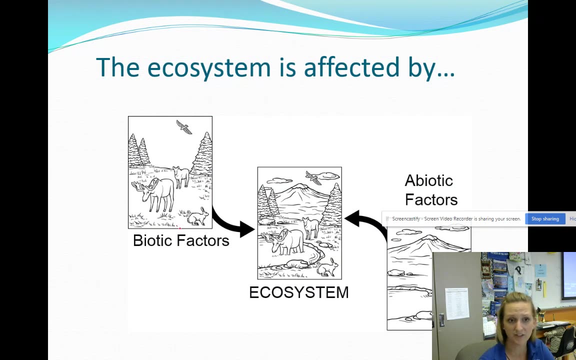 temperature is very cold. It has a lot of oxygen content dissolved in the water because it's just cold. It has high salinity. So those would be just a quick example of that. Okay, And so what's going to affect our ecosystem is the biotic factors, the living components. you know what you? 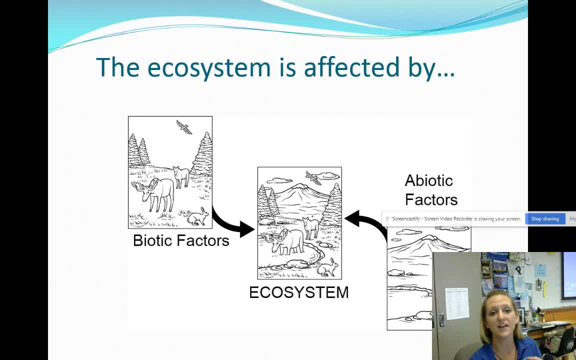 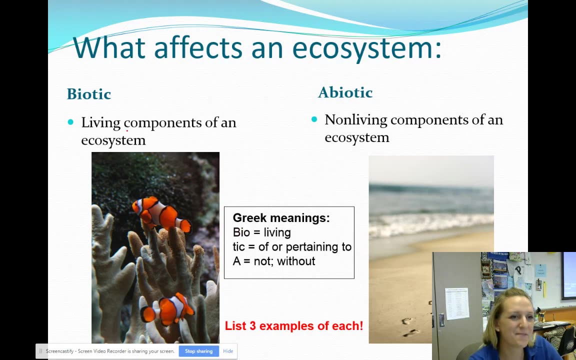 can eat? who you can mate with? Do you have competition with something? And then the abiotic factors, your non-living components. One, There we go. Biotic means living, So right here in the middle we have the Greek words: Bio is living, Tic means to be. 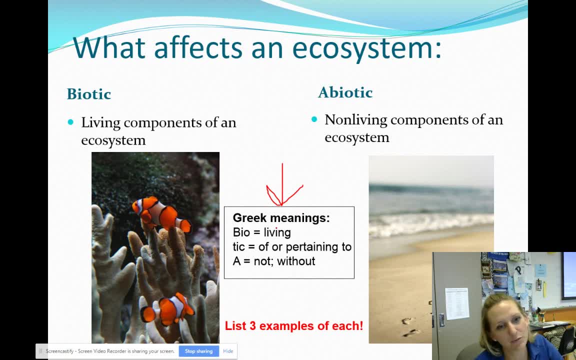 pertaining to. So biotic is pertaining to life And abiotic is not pertaining to life, Biotic or living components. Sometimes it's hard for students to think about that, but it's going to be predation, So that is a living component. a predator hunting a prey. 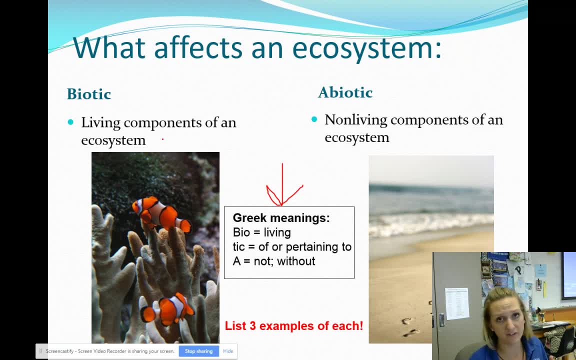 Symbiosis is a living component. Having a relationship, whether it's mutualistic, parasitistic or commensalistic doesn't matter, Having that inter-population or inter-species relationship. Availability of mates is a living biotic component. Availability of food is a living biotic component. We can't say availability of habitats because depending on where you live, it might not be a living component. 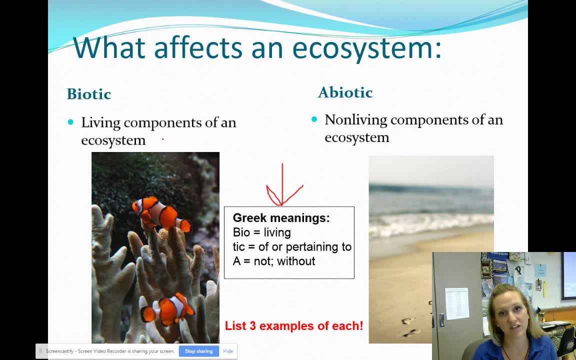 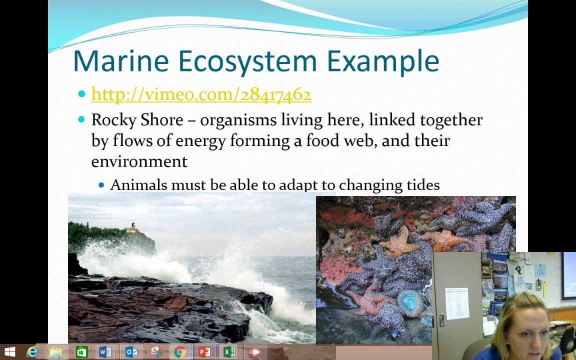 Okay, Abiotic is non-living. So again, what's the temperature like? What's the soil condition? What's the water temperature, The weather all the time? That's your non-living component, the abiotic. Okay, Let me pause One second. Okay, 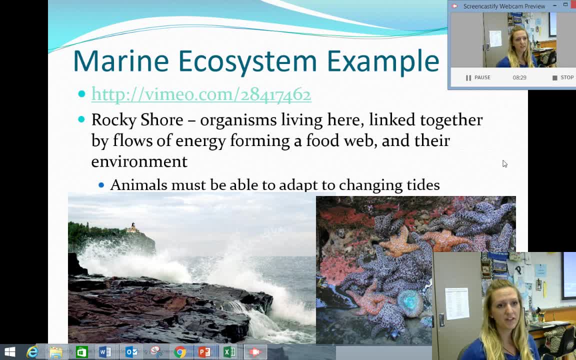 We're back. So a marine ecosystem example would be like a rocky shore. So it's going to be the organisms that are living there And they're linked together with their flow of energy, kind of like a trophic level transfer. who eats who? who's dependent on who? and their environment. So a lot of abiotic factors here are. you have the tide change, So you have some organisms that are exposed once the tide goes out. You have a very rocky substrate. 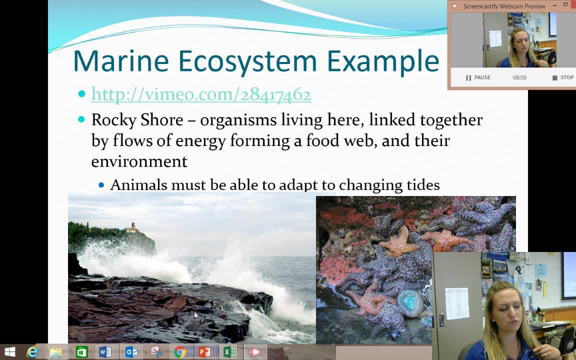 You see that word substrate. Substrate is the surface in which you grow on, So a sandy substrate, a rocky substrate, a marsh or mud substrate. The waves get quite big there. Okay, Weathering is high, There's a lot of weathering, And so that's just some of the abiotic components for that ecosystem, And the organisms there really have to be adapted to the changing tides So they don't want to dry out. And the fancy word, the Cambridge term for that, is abiotic. 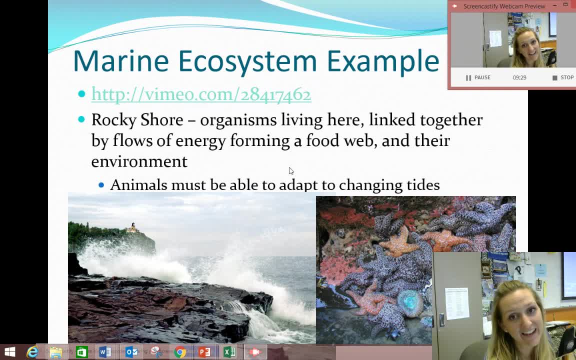 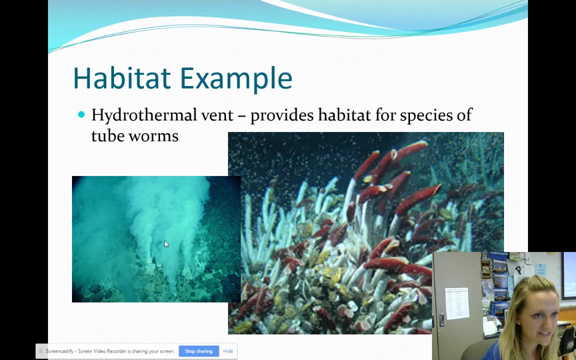 Okay, Okay, Okay, Okay. Okay, for dry out is called desiccate or desiccation desiccate. This video is funny. It's just a good example of some marine environments. Okay, habitat. example would be a hydrothermal vent. 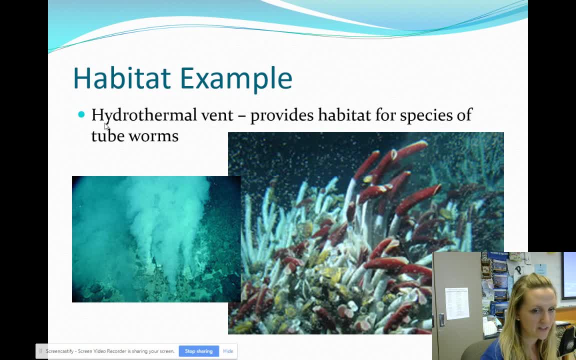 hydrothermal super heated water- It's the bottom of the ocean- provides a habitat for species of tube worms. The species of tube worm is called Riftia Riftia R-I-F-T-I-A Riftia. They live in hydrothermal vents. 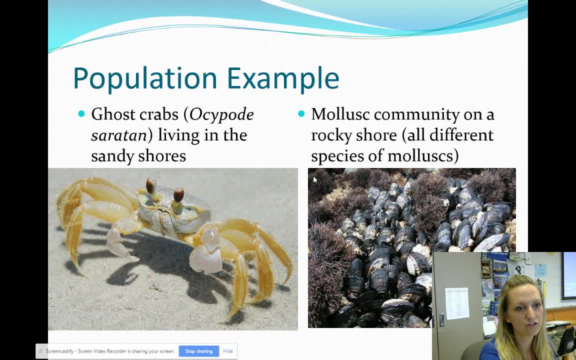 A population, so a group of ghost crabs live on sandy shores. Okay, and again, I just wanna real quick point out if we were trying to do population sampling with these ghost crabs, they move. So maybe mark and recapture might be something. 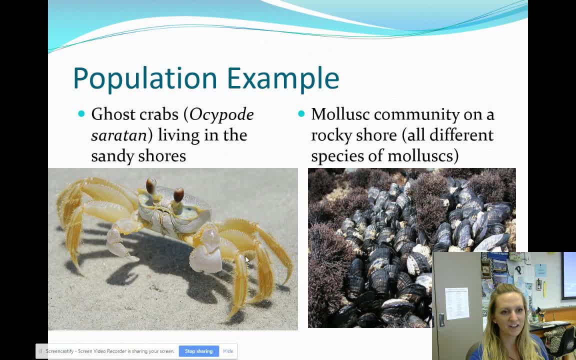 you wanna look at. However, the sky is really good at camouflage, obviously, A lot of times. the only time we see crabs at the beach is when we see them move, But imagine you put a dark color on this crab, something that will be evident to you. 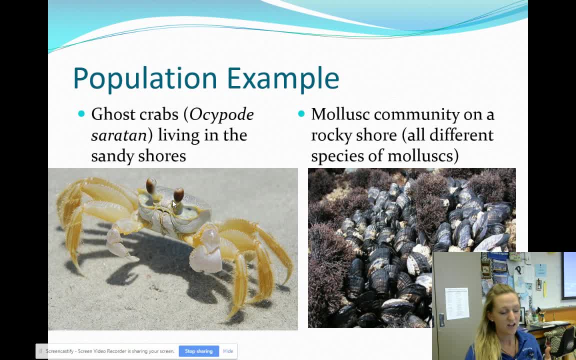 that's gonna cause that crab to be more susceptible to predation. It could harm it, it could wash off, and then you don't know who's in your original population And you're gonna have a bias The next time you go out there. 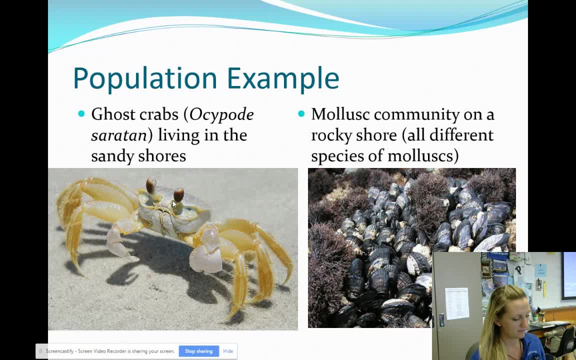 if you see a crab with a mark on it, you're gonna take it. Somebody else could take it too. So a mollusk community on a rocky shore, All different species of mollusk living here, Some small ones that you don't see. 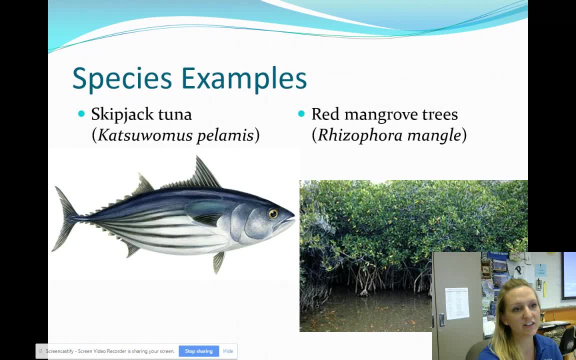 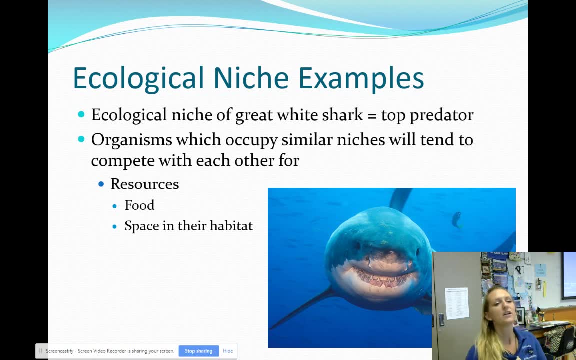 They usually grow on top of each other Species. example: a skipjack tuna or red mangrove trees, An ecological niche example. So this is the organism's role. So a great white shark, its role is to be an apex predator, the top predator in its ecosystem. 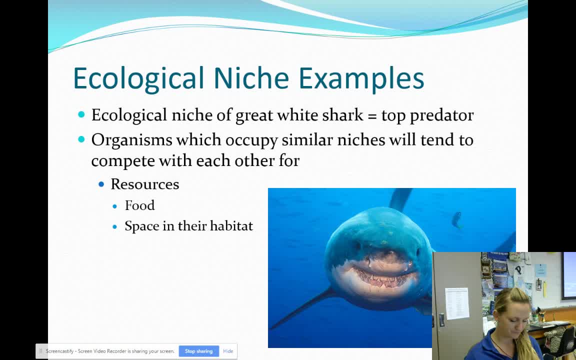 And in biology we talked about the competitive exclusion example, or, I'm sorry, competitive exclusion principle, an example principle. So that means that no two species, so two of the same, can live in the same habitat, doing the same role or the same niche at the same time. 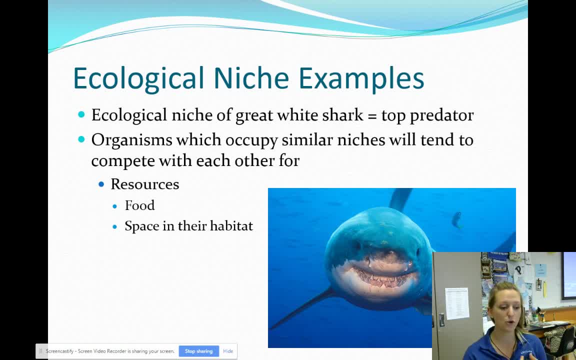 or else they will have competition. So one will have to leave or one will have to die, And that's the competitive exclusion principle. No two species can live in the same habitat, doing the same thing or the same role, the same niche, at the same time. 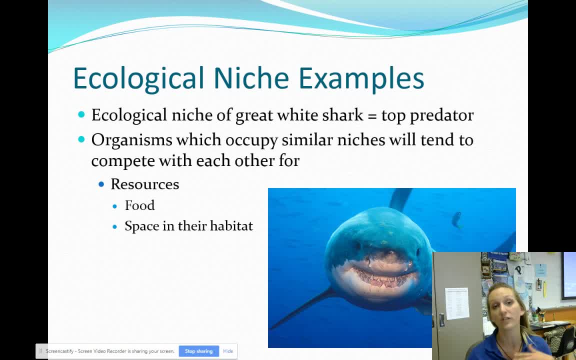 or somebody's gonna have to leave and someone's gonna have to die, or someone has to die, Okay, so the shark has its niche, And if something else came to take its niche, the shark would obviously try and kill it or get it out of there. 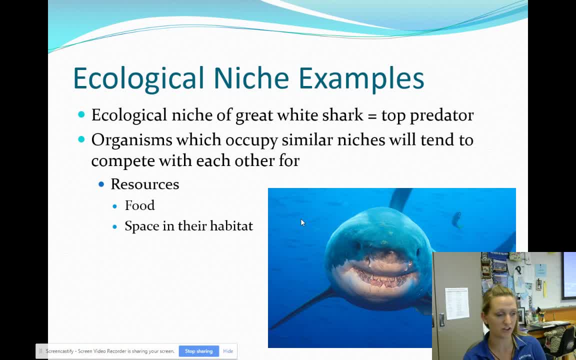 So organisms will occupy similar niches. They will tend to compete with each other. They're gonna compete for mates. They're gonna compete for ABs, for space. They're going to compete for food resources. If it's a land animal, they're going. 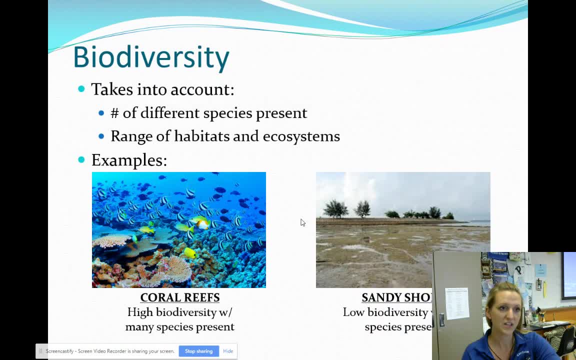 to compete for water resources. Okay, The term biodiversity, So bio is life, So this is going to be the amount of different species present in the ecosystem. Okay, And they do take into account the different ecosystems that are in that area, But this is the amount of different species in. 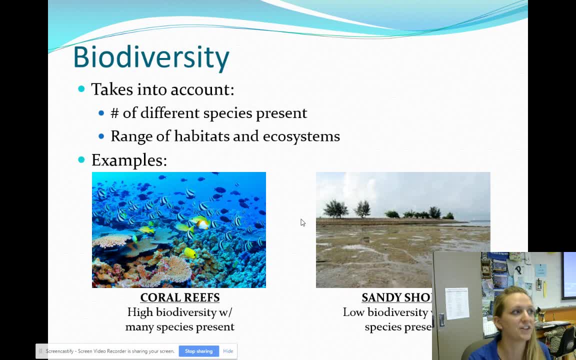 that area. Okay, So places that are very diverse are going to be rainforest, But if we're going to make it a marine example, coral reefs right. They have really high biodiversity, So many different species live there. We use coral reefs heavily whenever we're looking at new medicines, especially. 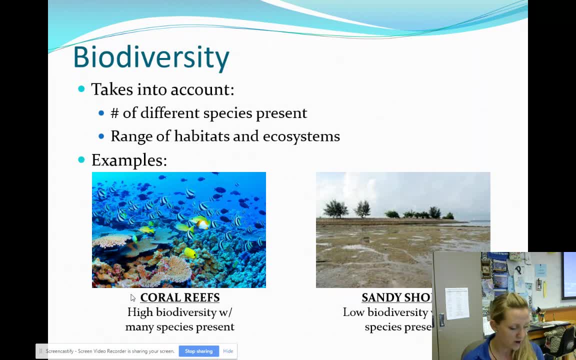 within the producers. They are the rainforest of the ocean. essentially Very high biodiversity, A sandy shore, Low biodiversity. There are not many organisms that can live within the sand- That many at all- Because they have to be able to adapt to being underwater occasionally and then exposed and out against the elements. 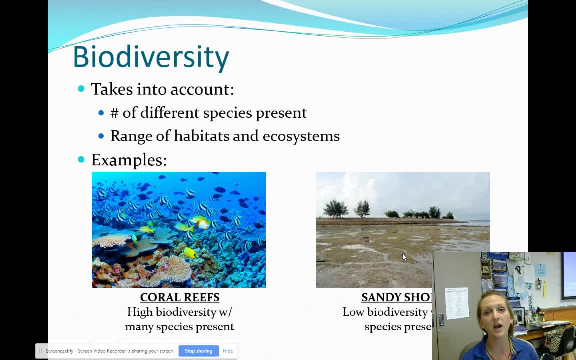 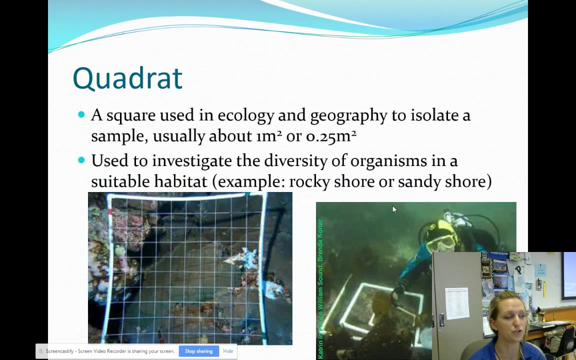 against the sun, against the cold, against rain, against predators. They have to find a way to burrow or find a way to hide, So that you know we don't really see many species or many organisms that are living in sandy shores. Okay, A quadrat Again. this is what we use to. 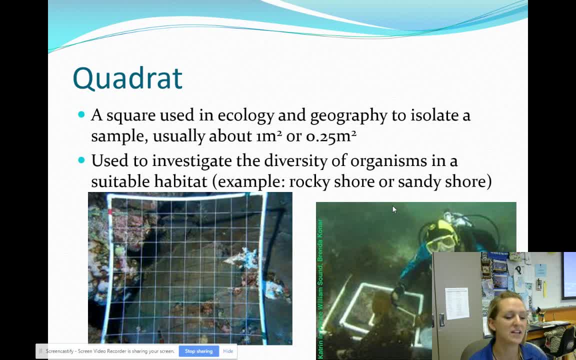 find a population estimate when we're using random sampling. So I noticed this a couple times when I was looking at the common cockle assignment. So a couple people are writing. I'm going to use the quadrat method, So it's really called the random sampling method. 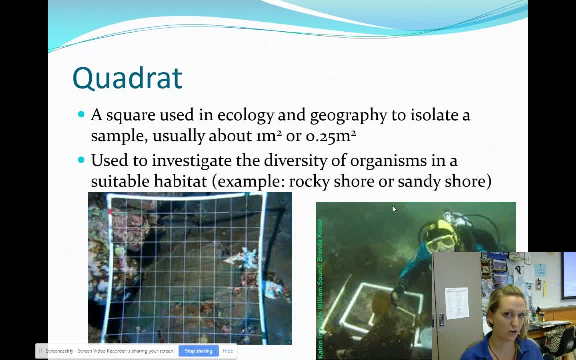 And you're taking a random sample by using a quadrat. It can be anywhere from one meter square large or a quarter of a meter square large, And you're taking a random sample by using a quadrat. A quarter of a meter square small. Okay, And this is going to be for organisms that typically don't. 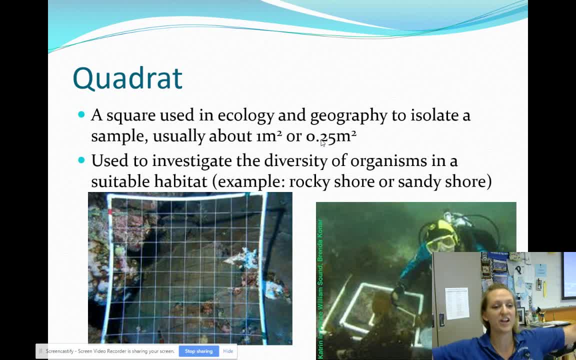 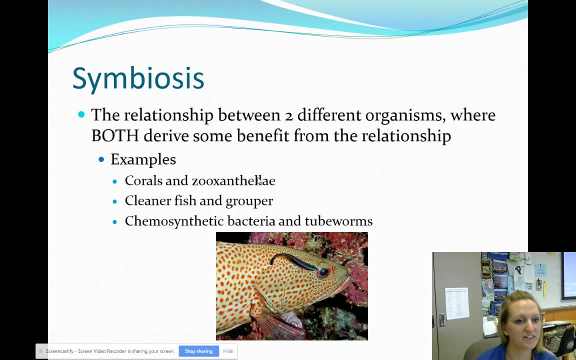 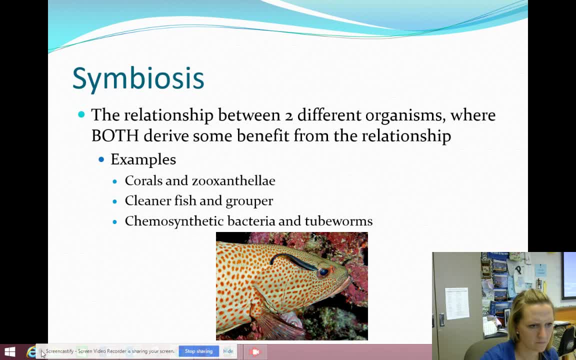 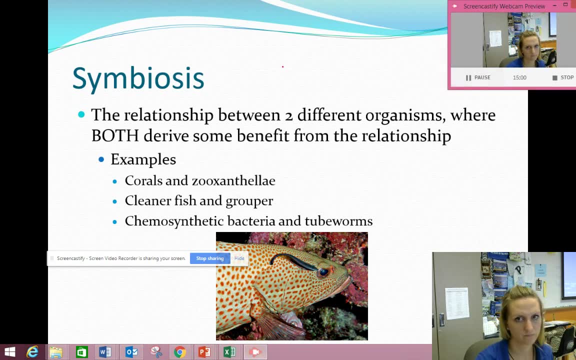 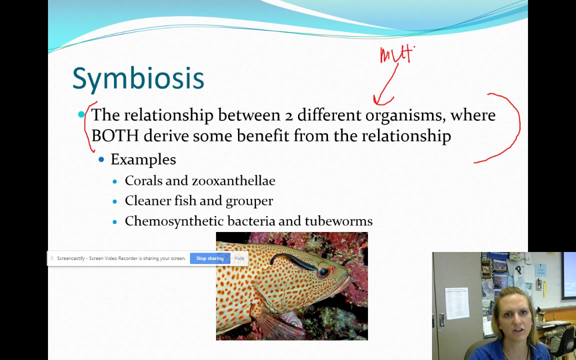 I don't know if it's pausing, Come on, Okay, Big mistake here. So symbiosis, This is not going to be your definition. This is the definition for mutualism. Sorry, This is mutualism. It's a cursive S Okay, Because this says both are deriving a benefit. The relationship between: 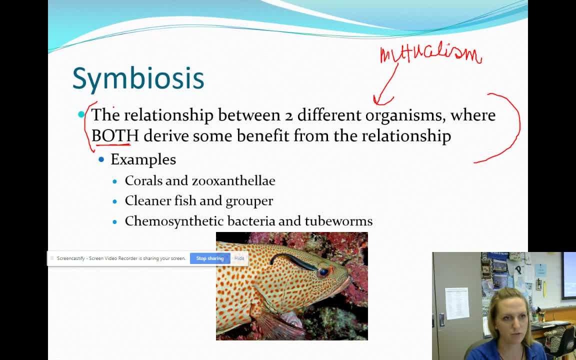 two different organisms where both derive a benefit. This is mutualism, Symbiosis. I'll just read it out of the text: Symbiosis literally means living together. The term refers to the interspecies relationship between two or more organisms from different species living in close. 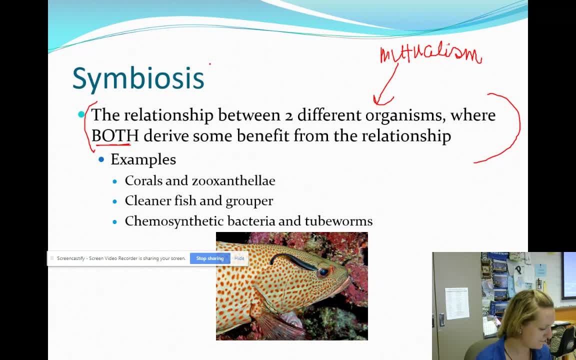 physical association. Okay, So symbiosis. Symbiosis is just having a relationship with something. Whether it's good or bad, it doesn't matter. That's what symbiosis is. So I'm really annoyed at that. This should be mutualism. Okay, It's your. 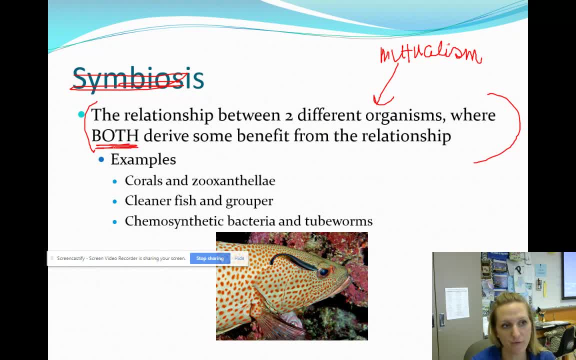 definition for mutualism: Both. So the relationship is mutual. There's both a beneficial factor. Excuse me, Okay, Examples are going to be corals and zooxanthellas. You have to know this one, You have to know this. 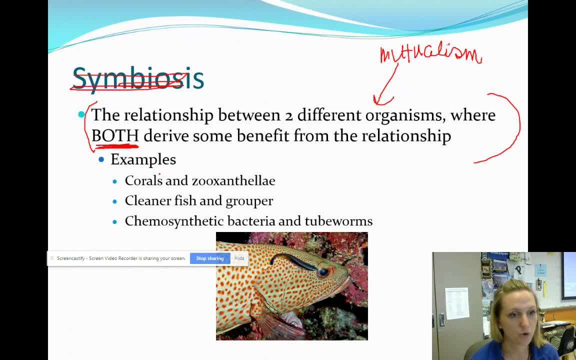 Cleaner fish and a grouper Or cleaner fish and any fish That cleaner fish- it's actually called a wrass fish, W-R-A-S-S. Wrass fish. Okay, Chemosynthetic bacteria and tube worms. Write down all of these examples. 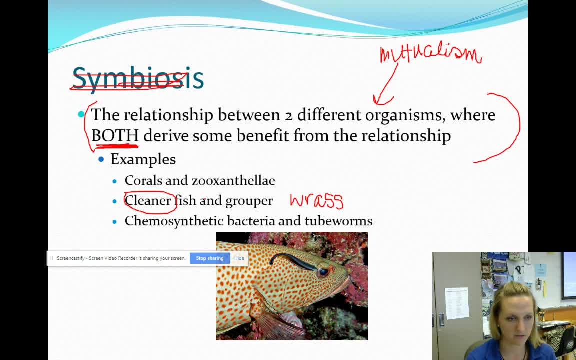 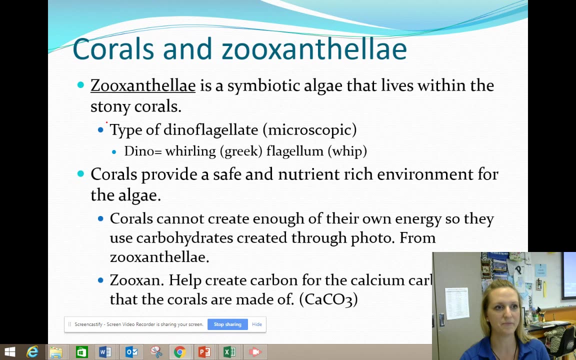 Write them down. Write them down All of the examples. You should be writing it down, Don't choose one, You need to know them all. Okay, So the corals and the zooxanthellae: You can say zooxanthellae, You can say zooxanthellae And, as you see, towards the bottom, I kind of got annoyed. 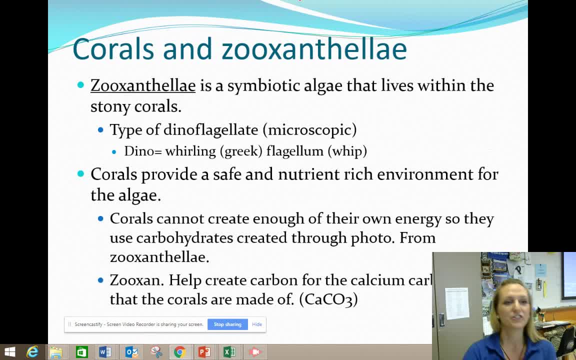 at typing it out, So I started to shorten it. Okay, So corals and zooxanthellae are a very popular question that Cambridge likes to ask about symbiosis. So zooxanthellae is a symbiotic algae that lives within stony corals- A symbiotic algae. 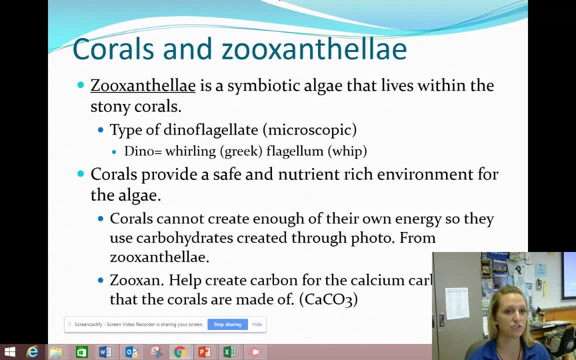 that lives within stony corals. So it's doing a job. It has a relationship with the corals. Okay, It's a dinoflagellate. Dino means whirling, And then flagella, or flagellate is from the word. 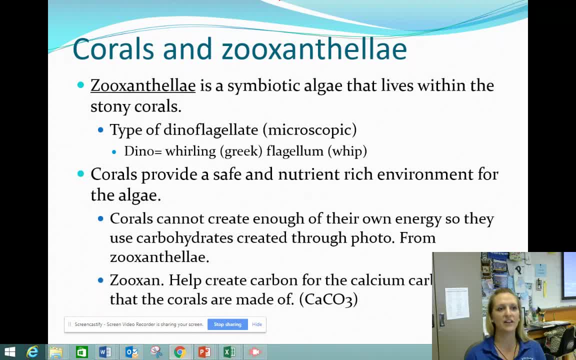 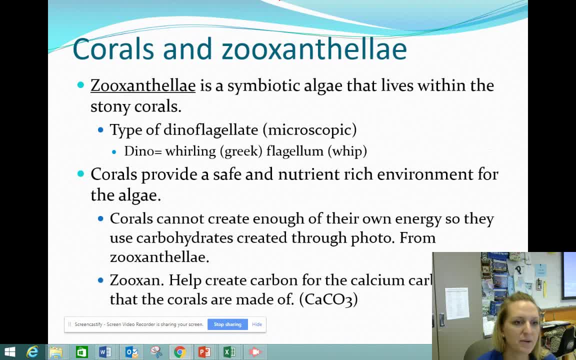 whirls, That goes in a circle. So how do they relate to each other? Corals provide a safe and nutrient-rich environment for the algae. Okay, So I'll- there's a couple on the side, and then I'll read a couple more that are a little bit more in depth. Corals cannot create their own energy, So 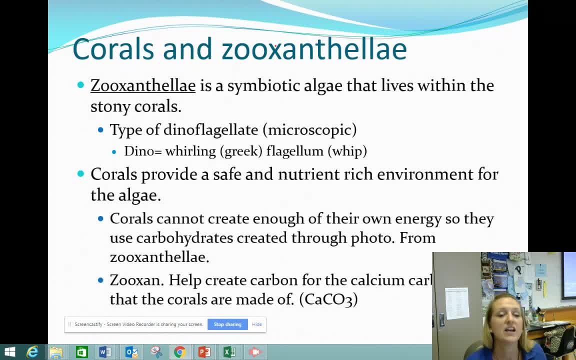 they use carbohydrates created through photosynthesis. It's the zooxanthellae. They are the algae, They are green. It's the zooxanthellae that is doing photosynthesis inside of the coral inside of it, And the coral is going to be able to. you know. 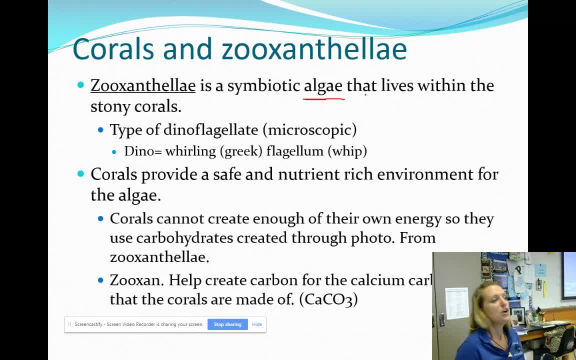 take some of that carbohydrates that are made and use it for itself. Corals are alive. However, they cannot make their own energy and they cannot get enough energy take in enough to keep them alive, So they have to. they have to have the zooxanthellae component to help them. Okay, Great, How do the zooxanthellae 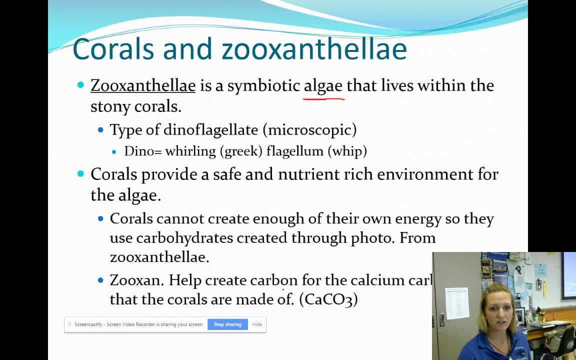 benefit. They help create carbon for the calcium carbonate that the corals are made of. All right, And I'll read a little bit more. So, as the coral grows, it respires aerobically and it will also. that will also provide the zooxanthellae. 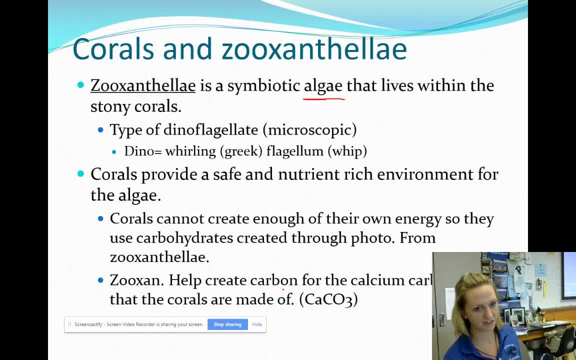 The zooxanthellae for carbon dioxide that it needs to do for photosynthesis. All living things are going to respire. The zooxanthellae is also going to respire. The corals also respire. Okay, The carbon from the zooxanthellae gets incorporated here in this calcium carbonate shell. 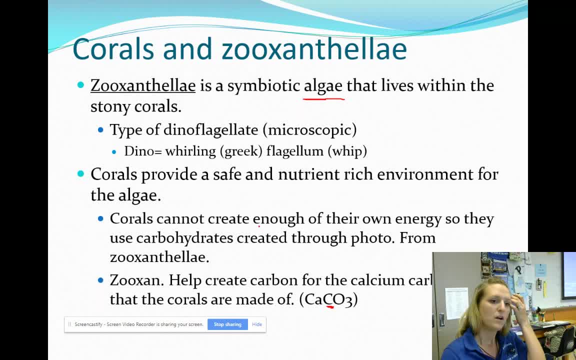 All shells are made of calcium carbonate. The last one, the zooxanthellae, provide a safe habitat with a big surface area so it can absorb light. They're provided with that. from the coral. The zooxanthellae also obtain other minerals. 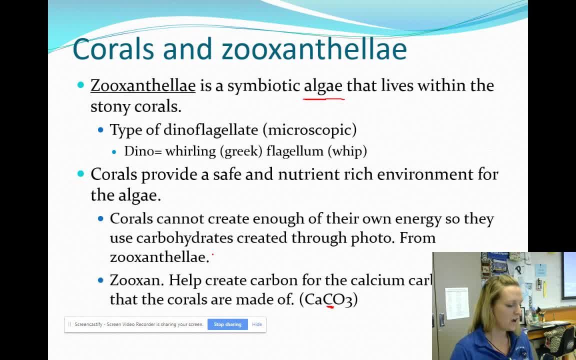 from the corals waste products, For example nitrogen compounds, so that they can make proteins and they can make ATP and they can make DNA. They also can use phosphates from the coral, The corals waste products, to create deoxyribonucleic acid, to make DNA, to make ATP: adenosine triphosphate. 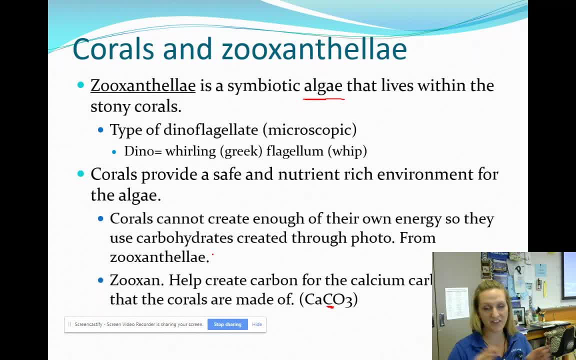 Also, the phosphates help on cell membranes as well that phospholipid membrane, So they both help each other in multiple ways. Test one a few times, watch the opposite side again, Listen to it again, pause it. write down what I have on the screen. write down what I just said. 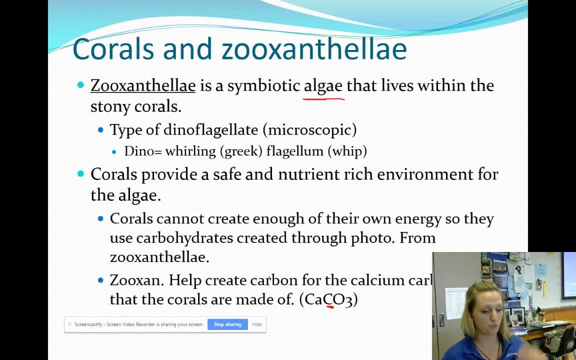 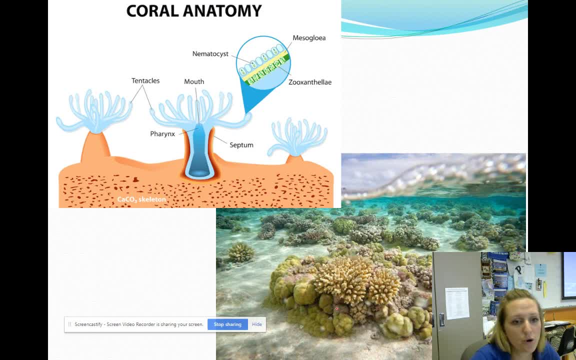 See if it's useful. Watch the next one. There is a little bit more information, a video if necessary, whatever you need. Here's what they look like. So corals- actually, you know they're a natural, like carbonate shell color. They're going to be like white And 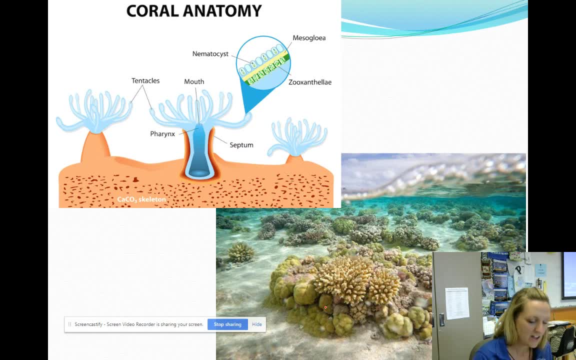 when we see color, you're actually seeing the zooxanthellae that live inside of it. So if we look at a coral anatomy- and you don't need to know the coral anatomy, but it should help you understand- They have this calcium carbonate skeleton. Calcium carbonate is kind. 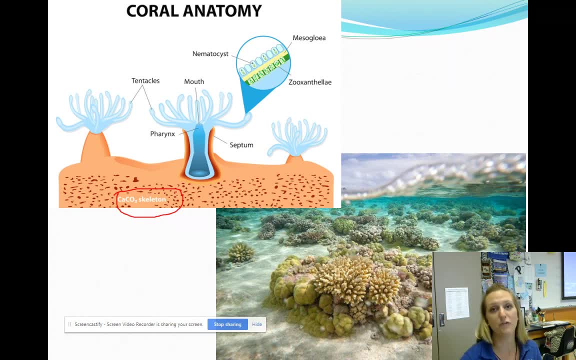 of like chalk, but it's harder. This is why they can dissolve whenever it gets acidic. All right, Looking at right at the edge of their tentacles. Okay, here's their mouth, so they can eat, But here's the edge of their tentacles And, like I said, they don't take. 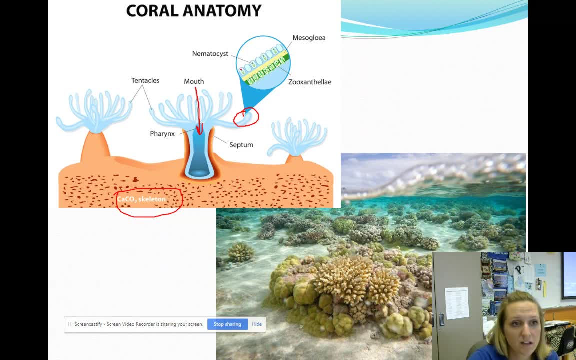 in enough energy through eating. If we zoom in On the outside, we have these little cells. They're called nomadocytes And what's inside of them is a nomadocyst, like a stinging. It's like a needle, And that's why some corals. 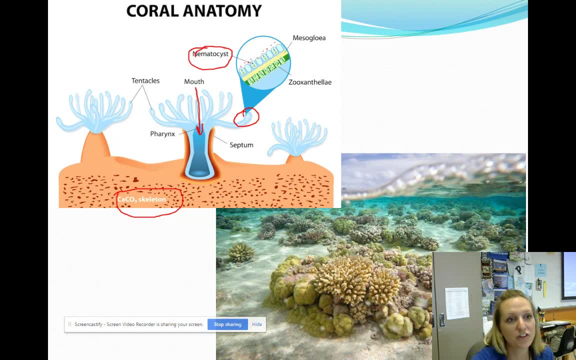 can sting you. Jellyfish also have nomadocytes. Remember, cyto is cell, So these are stinging cells. And what stings you is this tiny little, almost microscopic dagger. It's called a nomadocyst. Okay, Underneath that tissue is where the zooxanthellae live When corals are young. 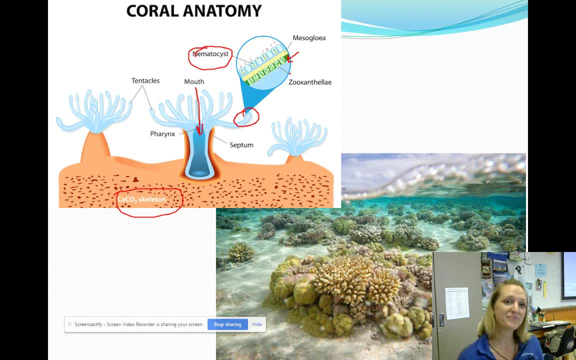 they like suck in these zooxanthellae and then they assimilate them into their body tissues, And so the zooxanthellae of course need to be on the outside of the tentacle so that they can take in all of the sunlight that they can, because they're photosynthesizers. 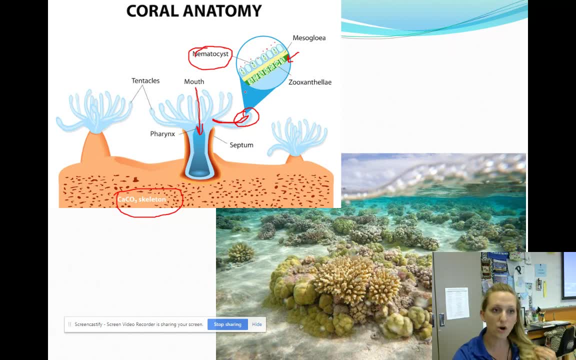 And their photosynthesis also helps the corals. Corals have energy and have a carbohydrate source, So corals and zooxanthellae are completely separate. They're besties, but they are completely separate If you see a color associated with. 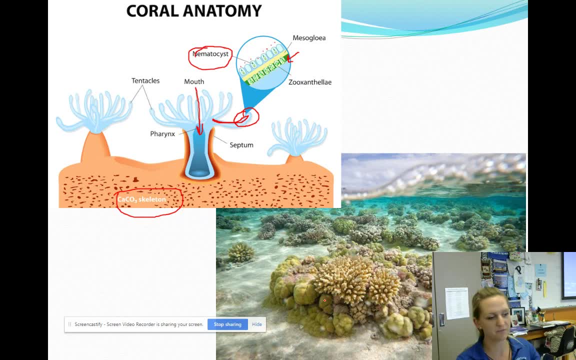 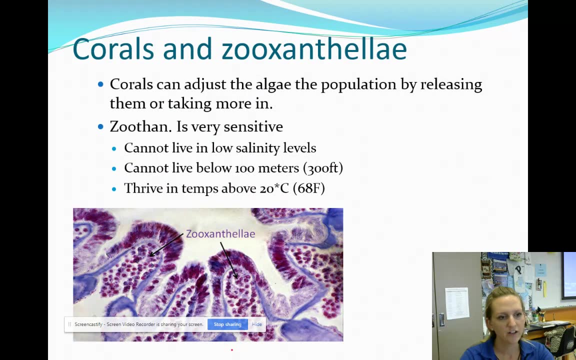 a coral. you are seeing pigments from the zooxanthellae. They don't just have chlorophyll. That's their primary pigment for photosynthesis, but that's not all they have Here. we can see it under a microscope. 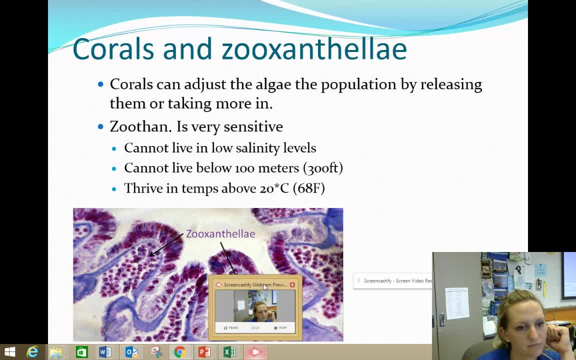 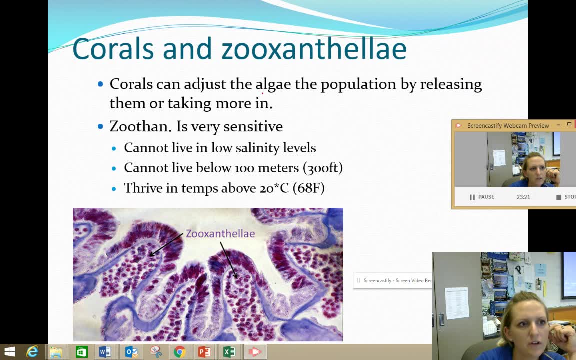 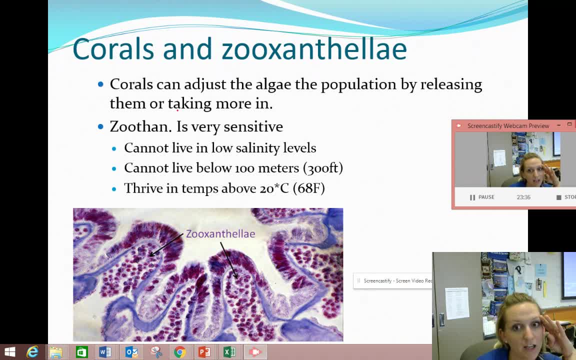 corals will eject out the zooxanthellae and be like you can't live here anymore, And that's why they start to bleach, because they lose their pigment, They lose theirmoke, Told you So. zooxanthellae is very sensitive, really sensitive. It cannot live in low salinity. 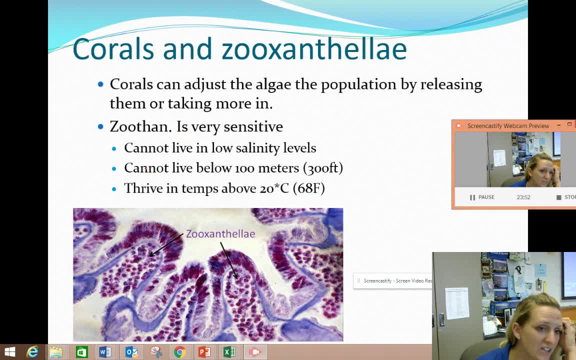 levels. So you can't have freshwater corals, Um, and that just helps with it doing active transport, passive transport, osmosis, Um, they cannot live below a hundred meters or 300 feet. Why? Because then you're out of the photic zone, you're out of the light zone, and they need to. 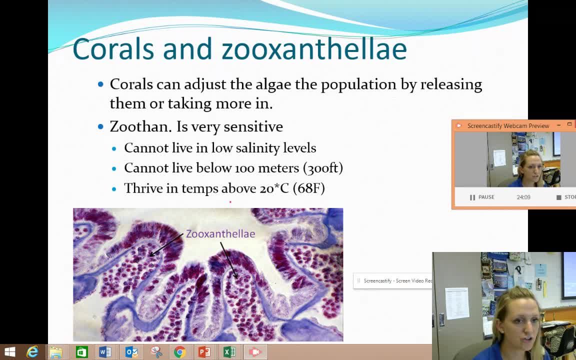 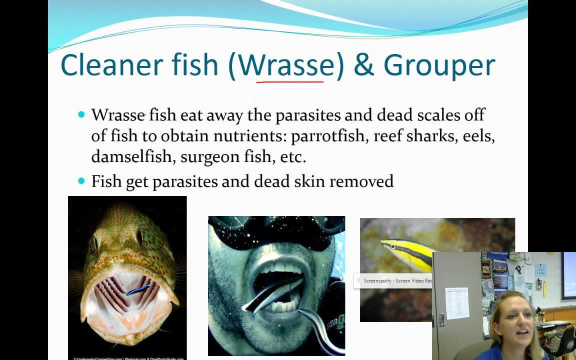 photosynthesize Um, and then they thrive in temperatures above 20 degrees Celsius, which is above 68 degrees Fahrenheit. They thrive above it. So this is like their threshold for their minimum. warmer is better. The wrasse fish. there you go, And the grouper. So the wrasse fish. 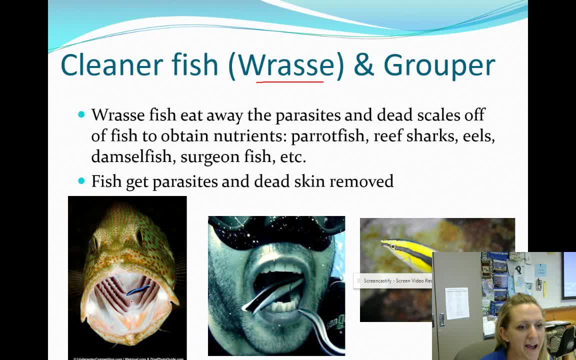 you guys have seen this before, especially if I was your teacher. Um the wrasse fish will go into the mouth of another organism and pick out um dead, dead skin parasites, And they help keep the mouth clean of these organisms. 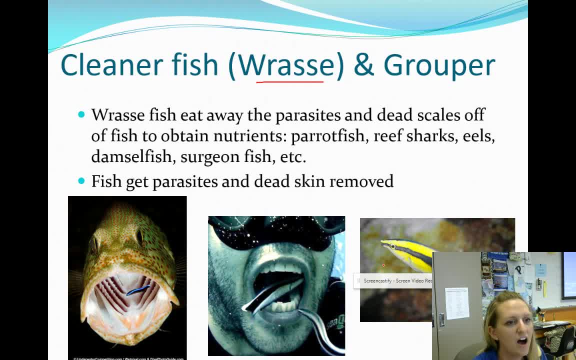 Fish don't have hands. They don't have a dentist. Um fish get parasites and dead skin removed. So the wrasse fish is your cleaner fish And that benefits by getting a nutrient source. Your grouper is going to benefit, or any other fish is going to benefit by getting their. 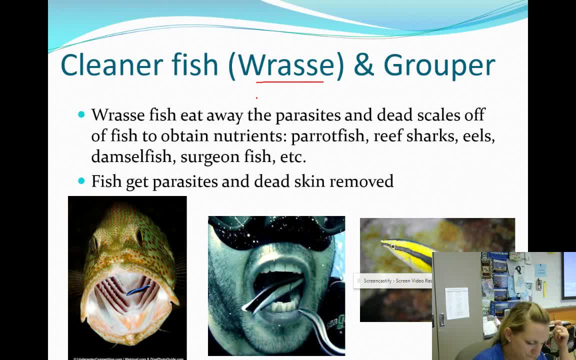 their mouth cleaned um, or parasites take it off? Um, if there's, yeah, that's fine. Sometimes there's parasites on the gills Taking it off, there is good, Um. there's a lot of examples of this: Pilot fish cleaning off sharks. 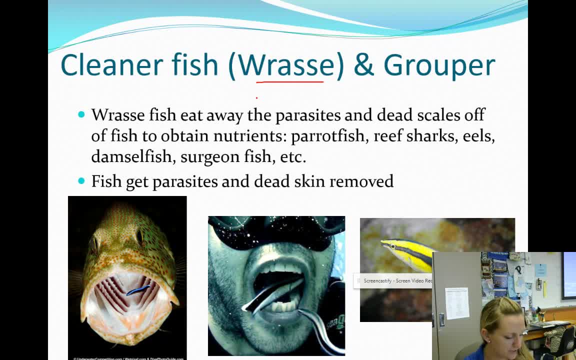 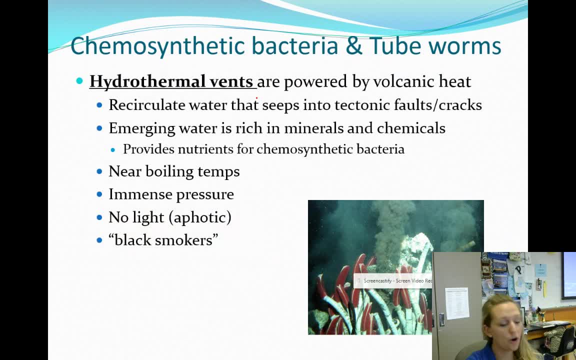 Pacific cleaner shrimp and blue streak cleaner wrasse cleaning eels. Okay, Know and understand chemosynthesis and these in this relationship- we're going to talk about chemosynthesis for a while- and it is a primary productivity source for the ocean, So 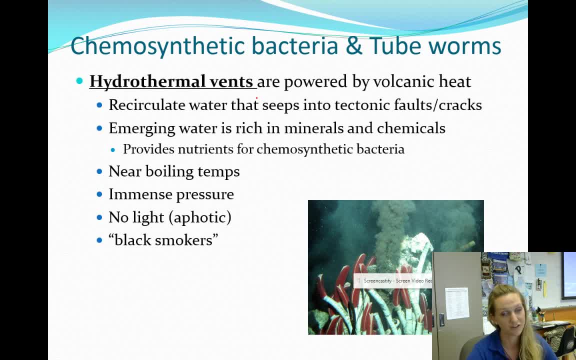 we can't ignore it just because we're like, oh, we're going to have to clean up the ocean. So, like more familiar with photosynthesis, we have to know this. So chemo means chemical and synthesis means to make. this is chemosynthetic bacteria. It is microscopic. 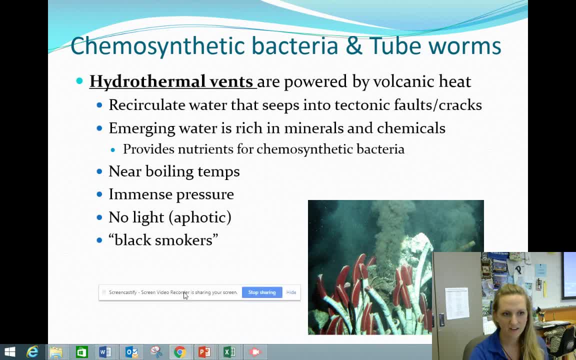 bacteria that live inside of these two worms. They live inside of them and they do this process called chemosynthesis. Chemosynthetic bacteria perform chemosynthesis Um plants, or autotrophs, photoautotrophs, perform photosynthesis, So the mutualistic 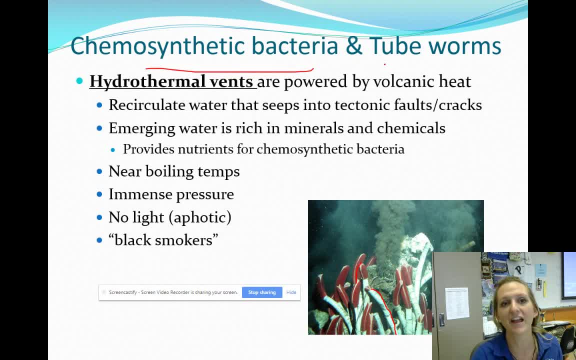 relationship organisms. here are the chemosynthetic bacteria and your tube worm. So a hydrothermal vent. hydro is water, Thermal is heat. These are vents powered by, like volcanic heat, from underneath the earth. The earth is not a, the earth is not flat number one, but the bottom of the ocean. 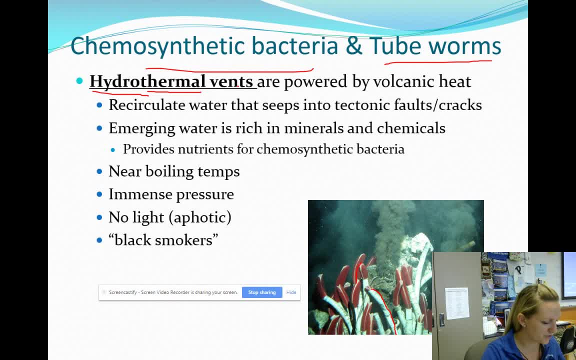 is not perfect, Um, the the lithosphere there does have some deformities and it does have some areas that are- um- what's the word? Vulnerable. So, for example, the lithosphere is not perfectly thick the whole way. you know, underneath your ocean You could have some areas that are thin. 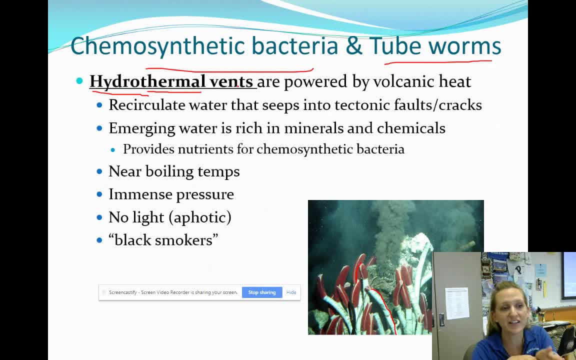 It's going to be those areas, or at plate boundaries, tectonic plate boundaries, that magma is going to push up. You know, the mantle of the earth has so much pressure built into it. Um, it's literally going to push out of any of that crack. Um, just because it's 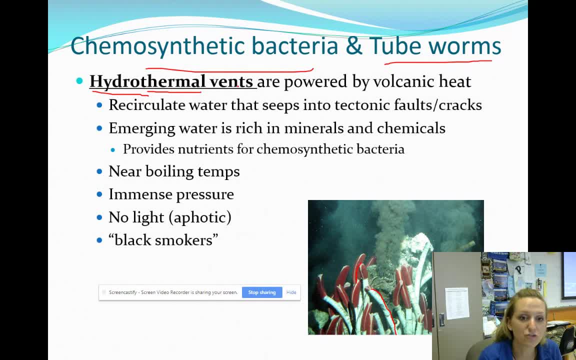 it's a vulnerable area, So that is where we can create these hydrothermal vents You there. sometimes they're called black smokers because they um release a black plume of gas. You can see it right here. Is this No Okay? 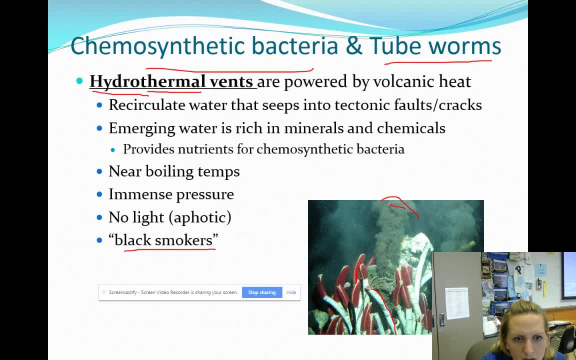 Is it a link? I'm sorry, I'm a poor soul at the moment. This is a link, Okay, So I mean you guys can go on the actual website, I believe or not? the actual website, actual PowerPoint and. 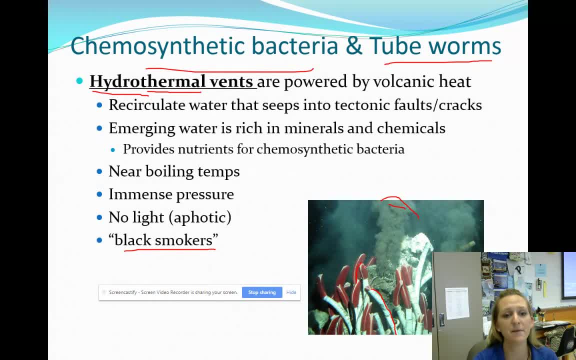 click this picture. It looks like it is Anyway. Um, you see this really big plume of black spoke. It's big, It's big. This picture doesn't give it justice, but that is tons and tons and tons of super hot water in dissolved 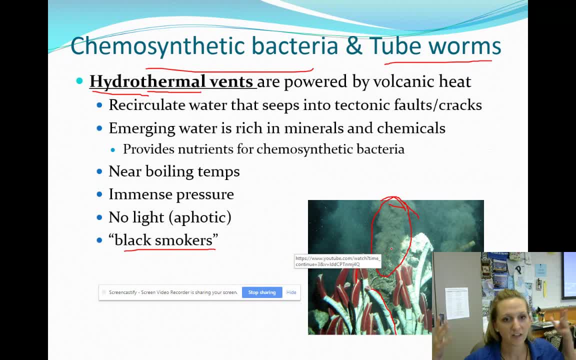 Minerals from the earth's crust coming out into the ocean. within there, um are a ton of different chemicals. We'll get to in just a moment. So what is the conditions like in this area? Um, we have water that's being recirculated. It will seep into the tectonic cracks and come back out with. 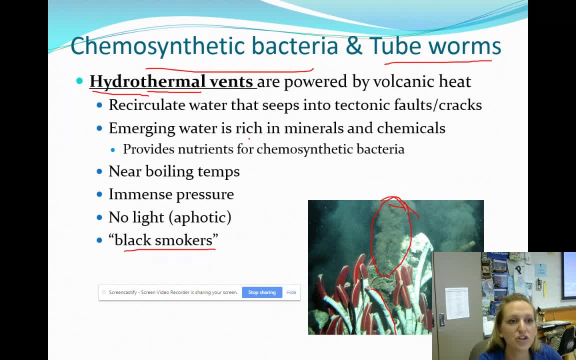 the pressure It gets like super boiled. The emerging water that comes out is rich in minerals and chemicals. It's going to provide the nutrients for photosynthetic or chemosynthetic bacteria. So photosynthesis, um the energy, for that is coming from the sun. Chemosynthesis, the energy. 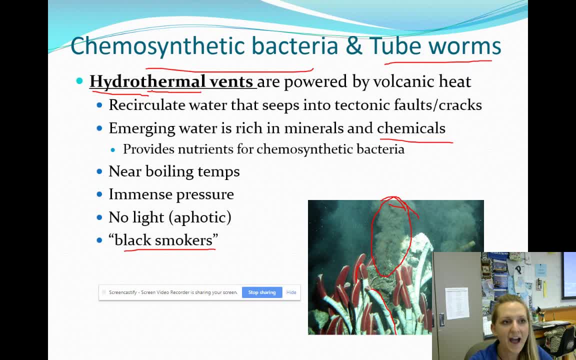 from. that is coming from chemicals that come out of these hydrothermal vents, And the chemicals are from the crust of the earth. You are near boiling temperatures here. So even though it's super cold down here and the pressure is immense, um, no sunlight shines there, So it's super cold. 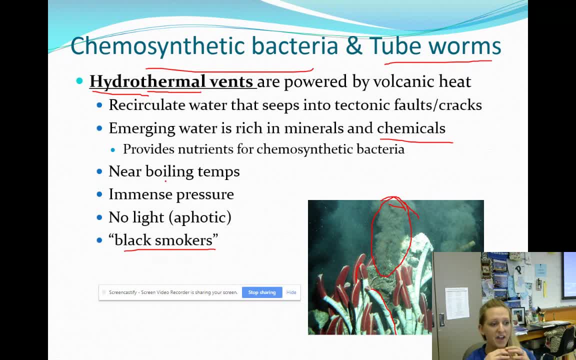 But it does get near boiling because, um, of the all of that energy coming from the mantle of the earth, Tons of pressure, Um, there's no light, and they are also called black smokers. These conditions, what it's like there, you need to know them. So let's talk about the actual. 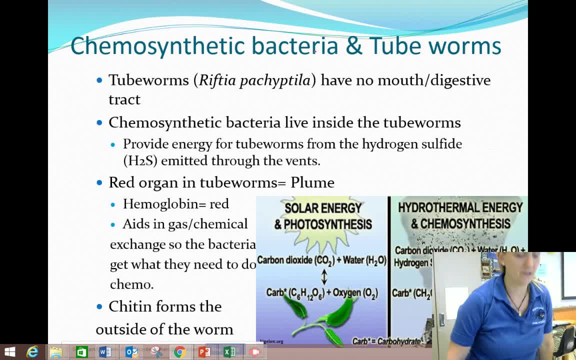 relationship. So what tubeworms? the tubeworm species is called Riftia, pachypteris Tila. We can call it Riftia. You need to know Riftia. So um Riftia, they don't have a mouth. 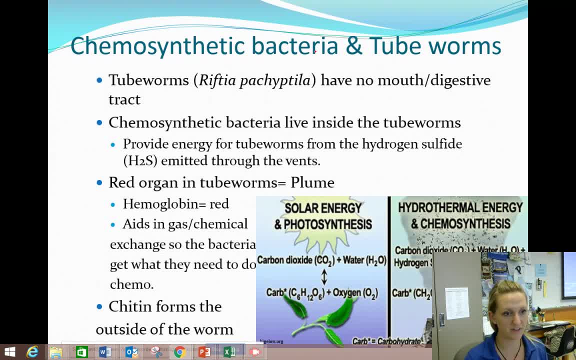 They don't have a digestive tract, So I'll talk about um on the next slide, I believe, how they get bacteria inside of them, Okay, Um. so inside of the tubeworms, just like inside our intestines and inside our stomach, we have um symbiotic bacteria that live in there, help break down. 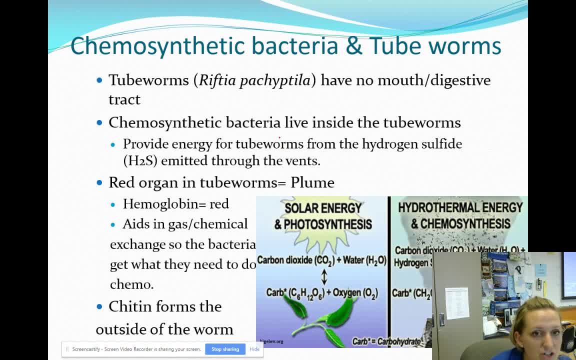 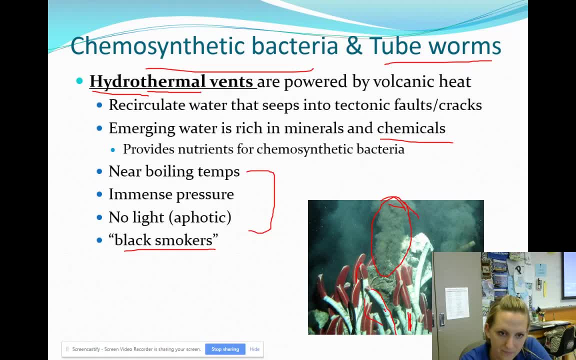 our food? Um chemosynthetic bacteria live inside the tubeworms. They live oops down here in the white area. The white area is called chitin. It's like um similar to keratin, but chitin is like. 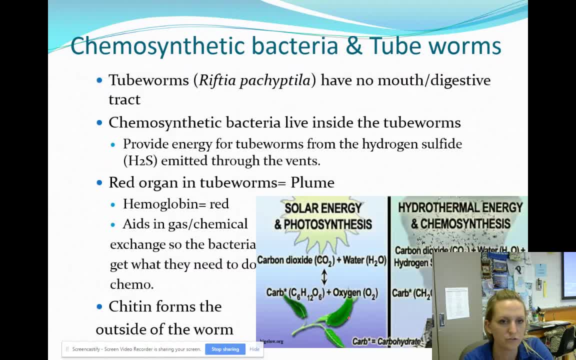 the exoskeleton of arthropods: a cockroach, a beetle, Those are chitin. Okay, So the chemosynthetic bacteria live inside the tubeworm. Awesome Tubeworm doesn't have a mouth or a digestive tract. 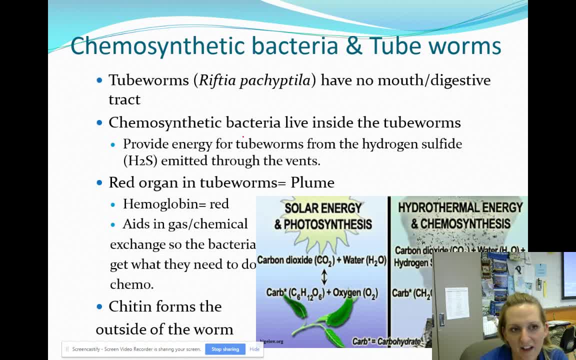 so it can't eat food itself. It's going to rely on this bacteria. Um, they provide energy for the tubeworms from hydrogen sulfide. hydrogen sulfide that comes from the vents Know this. So for photosynthesis, your energy component is sunlight. For chemosynthesis, your main energy. 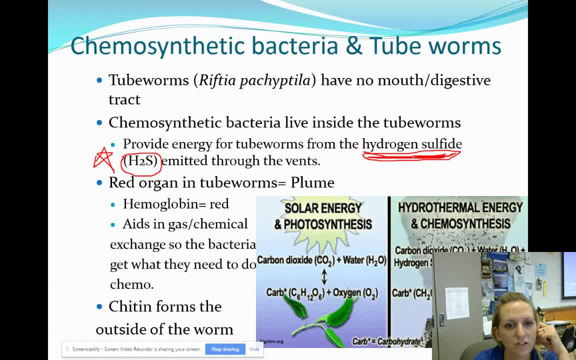 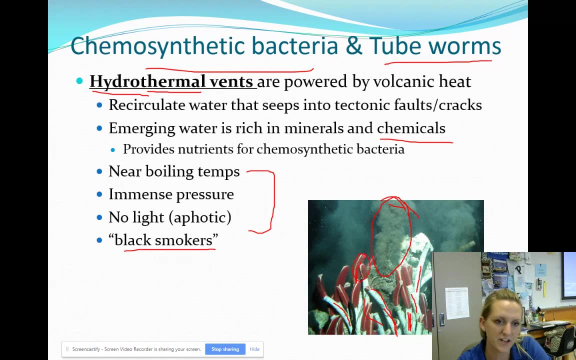 component is hydrogen sulfide. Hydrogen sulfide Smells really bad. Um, this is just supplemental. It's about the tubeworm. Um, the red organ you see in the tubeworm is called the plume, So this right here is the plume. 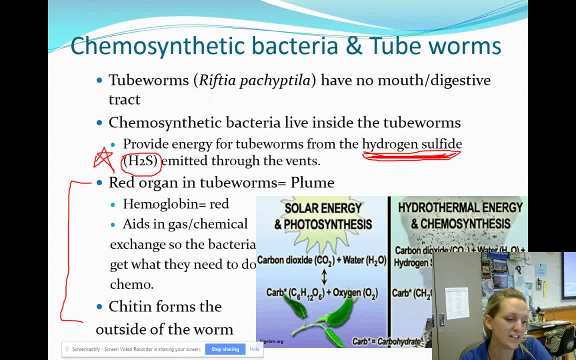 It's red because it has hemoglobin, which is the same protein that we have that takes oxygen around ourselves. So it aids in gas exchange, So the bacteria can get what they need to do to do chemosynthesis. Um, they need this gas to do chemosynthesis, So they need this gas to do. 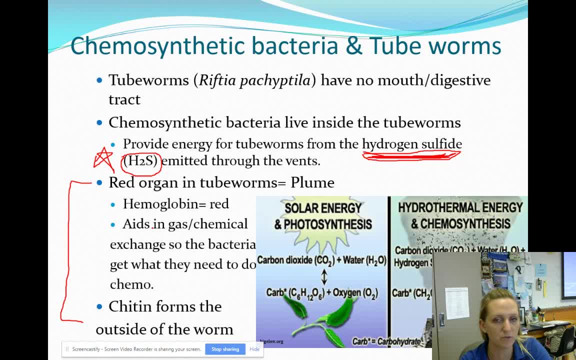 chemosynthesis. This hydrogen sulfide gas transported to them, Hemoglobin, will help do that. They also need um oxygen taken to them and carbon dioxide taken to them. All right, Um. and if we are looking here at the formula now, I think the idea of chemosynthesis 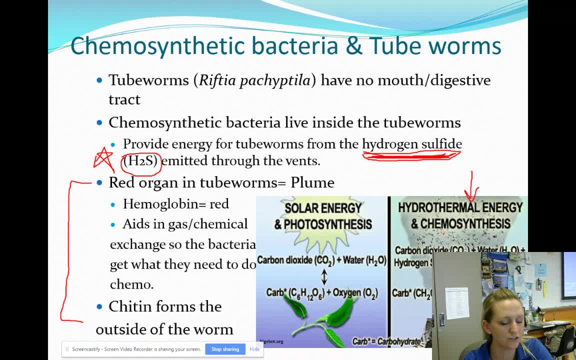 is pretty new for scientists, and still not 150% on the exact formula, because there's multiple ways they can chemosynthesize. So you see, um, there's different carbohydrates that can synthesize. carbohydrates are carbon hydrogen and oxygen in a one to two to one ratio. They also release. 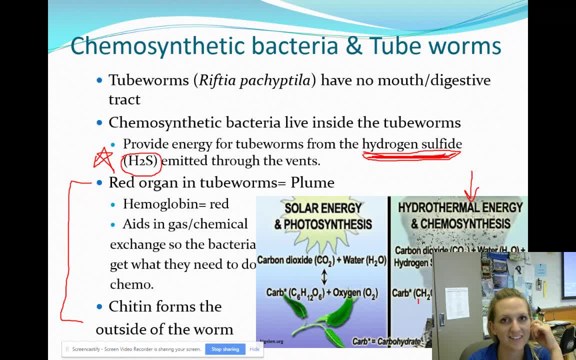 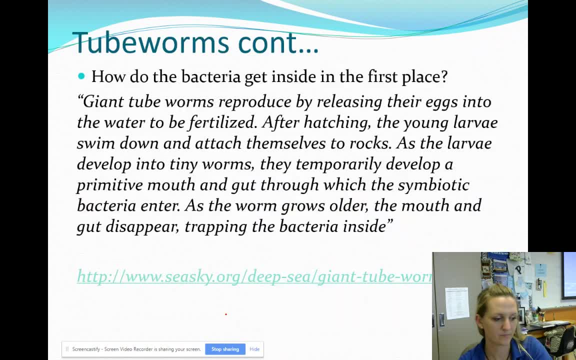 sulfuric acid. sulfuric acid. So that makes conditions in the hydrothermal event really acidic. But um, back to what I was saying, I've seen chemosynthesis formulas with multiple different energy sources, not necessarily always hydrogen sulfide. Um, it's really. 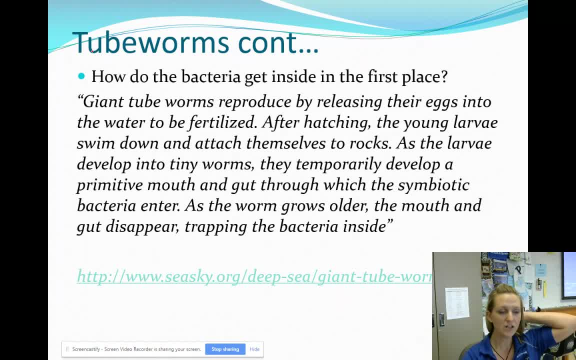 depending on what's coming out of the hydrothermal vents. Um. so how do our bacteria get inside of the tube worms in the first place? So when you just have a baby little tube worm, baby little Riftia, Riftia, Um so the giant tube worms reproduce, they release their eggs into the 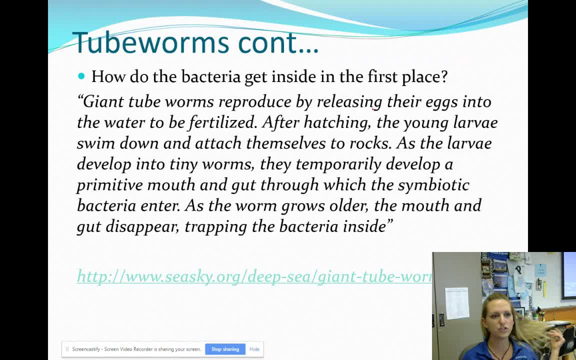 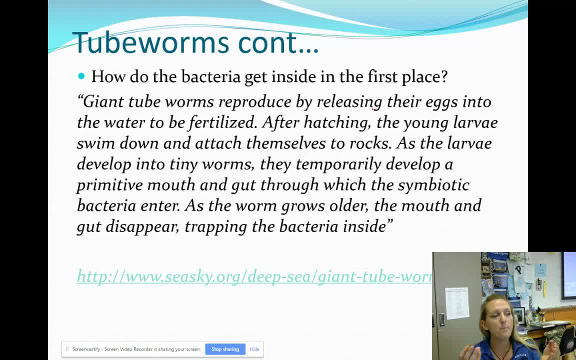 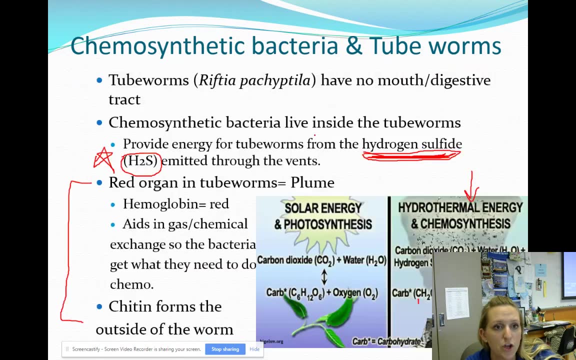 but as the larvae start to grow, they will make a um, just a temporary mouth and a gut, so that they can take in the symbiotic bacteria. If they don't, as adults they don't have mouths. no mouth here. no mouth. There's no mouth. no digestive tract. no mouth, no digestive tract. 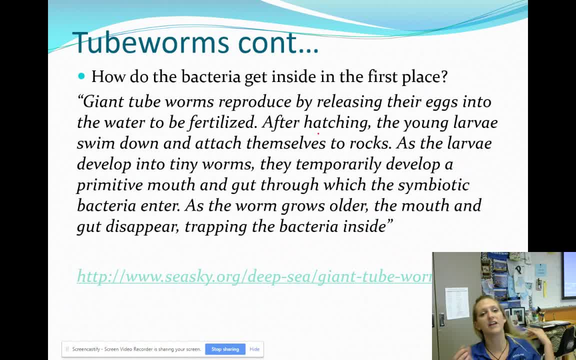 So they need a way to get food. in the very beginning of their life They have this tiny thing that they can suck in this bacteria. As the worm grows older, the mouth and gut go away and the bacteria get trapped inside. So where is it beneficial? Um the tube worm, the actual long 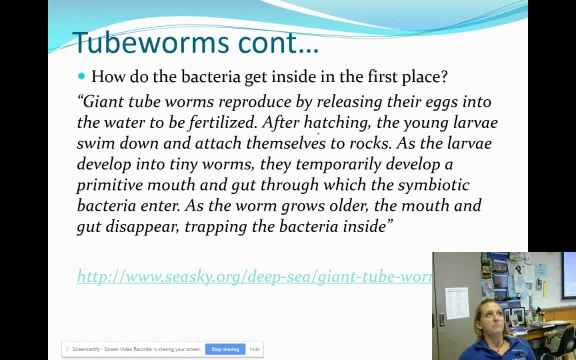 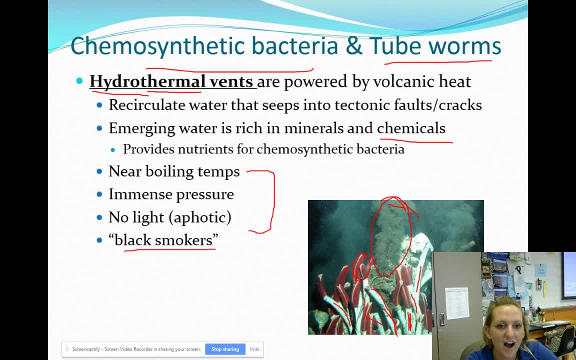 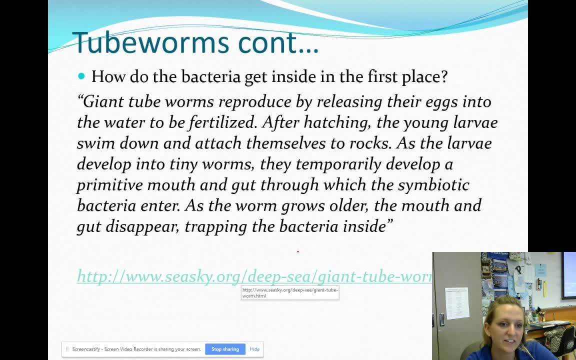 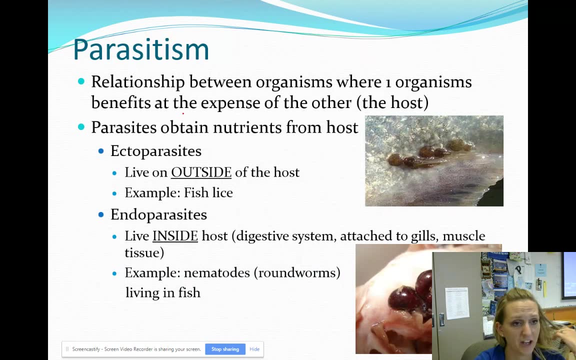 Now, these two worms live on the vents, So the bacteria need a place to live really close to the vents as well. Click this. There's just a little bit more information about the giant tube worms. Parasitism, So like a parasite, this is a relationship between organisms where one is 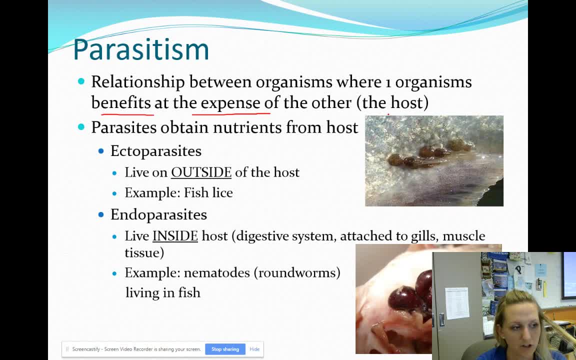 going to benefit at the expense of the other, the host. So the host is getting eaten and the parasite is doing the eating. Parasites are going to get their new job. Parasites are going to get transferred from the host. They can, um you know, transmit uh multiple diseases Um parasites. 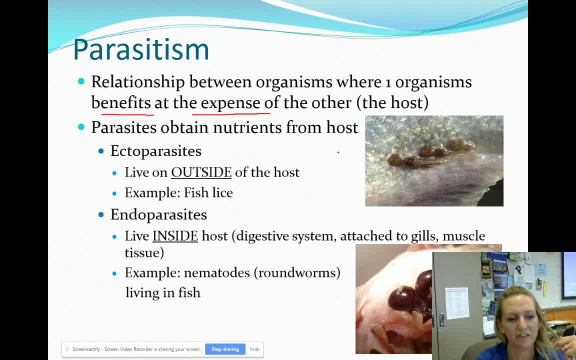 can lay their larvae eggs inside of your tissues and they'll live off your tissue. Two different kinds of parasites. One is ecto parasite. Ecto, Ecto means on the outside, So they live on the outside of the host. For us this would be like lice um, mosquitoes, fleas, ticks, fish. 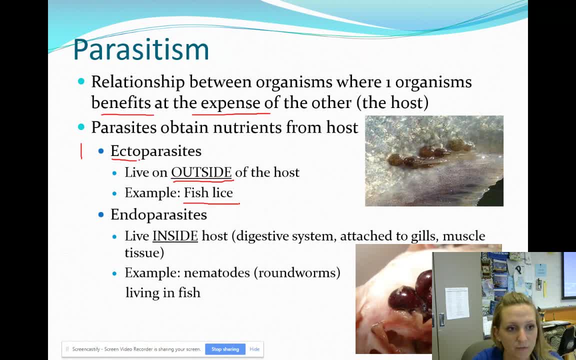 lice, That's an easy one to remember. Or um, sea lice, sea fleas- That's an easy one to remember. We see that a lot. So here they're, living on the outside of the scales. Endo parasite- um, like endoscopy. 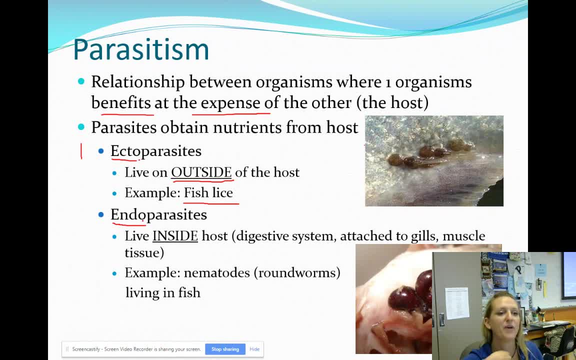 Endoscopy is when you swallow a camera and they and inside, So endo is inside. These are parasites that live inside of the host. They can live in the digestive system. They can attach themselves to gills, like you see in this picture. here, these hookworms. 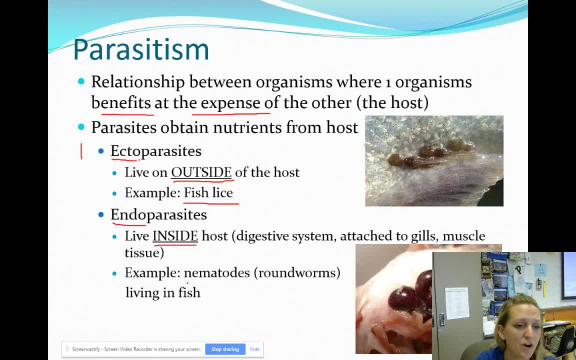 Um, they can live in muscle tissue. An example are Nema toads, or you can call them roundworms living in fish. There are multiple questions that say: give an example of um or describe what parasitism means and give an example from the marine environment. So you're pretty much. 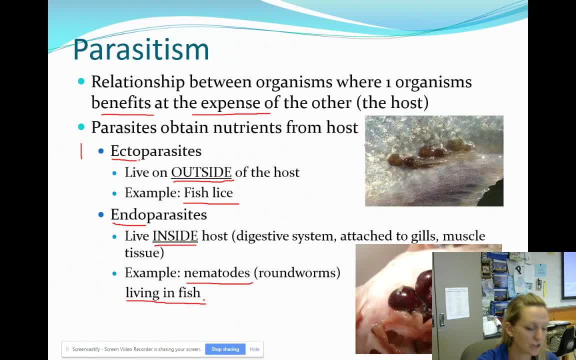 going to give the relationship and you're going to give an example from marine environment. You can say um worms, you know roundworms living in fish, Nema toads living in fish, fish, um fish life living on the outside of a grouper, like literally, pick one of these easy. 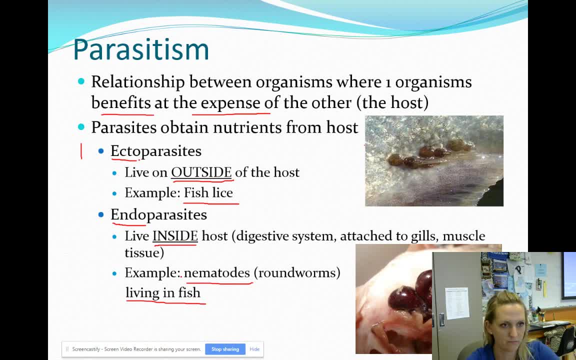 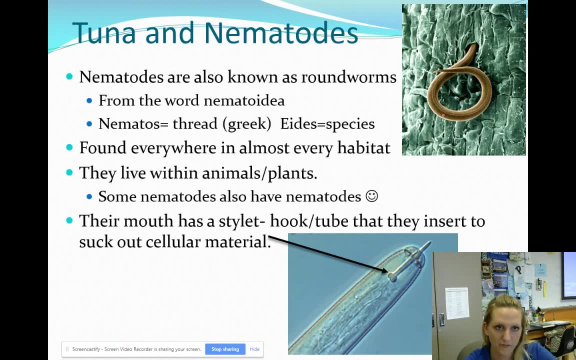 parasites and then an organism. They need to be marine, though. Here's your scanning electron microscope picture of a roundworm in the tissue of a fish. So Nema toads are from the Roman Nema toad. Nema toast means thread. It's tiny, tiny, tiny, and edase is species, So it's 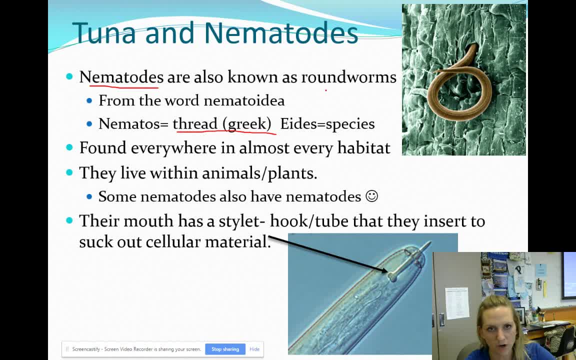 like a thread species, but they're also known as roundworms and they're tiny, Um. they are found everywhere, in almost every habitat. They are- I want to say like when the most, they are the most abundant parasite that, um, that the world has. They are in every. 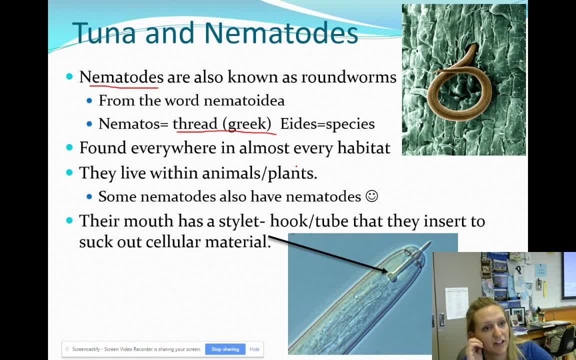 habitat and almost every organism they can live in, so they can live within plants and animals. Some Nema toads have their own Nema toads. I love that Some parasites have other parasites living in them. I just I think that's just awesome. 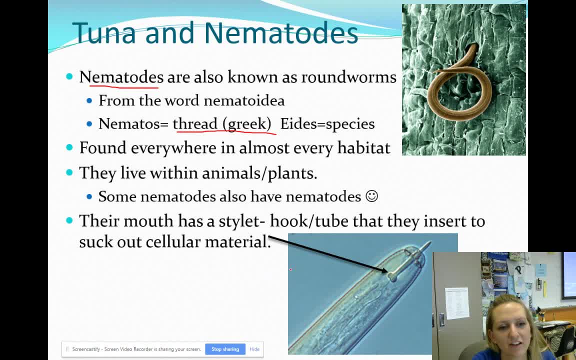 Nematodes. So, um, you don't need to know this just a little bit extra. Why not know it? Why not know everything? Um, their mouth has a stylet. They have a stylet. It's a hook, or like a tube. 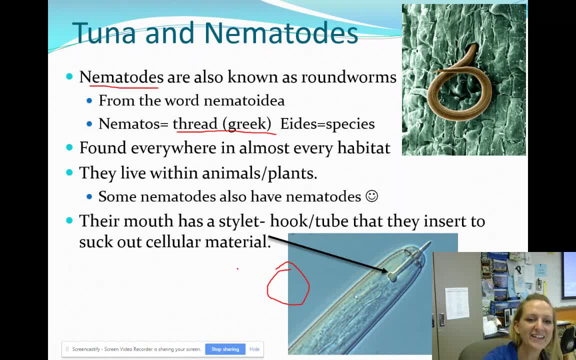 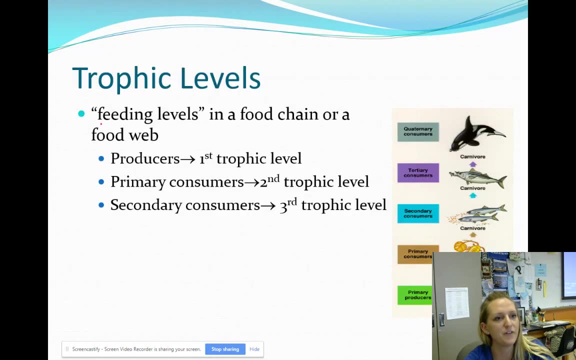 that they will insert into a cell and suck out cellular material. So this is microscopic. It's super small, super, super, super small. but nematodes have nematodes And an example could be nematodes and um tuna fish Trophic levels. Trophic literally means the feeder, So the feeder. 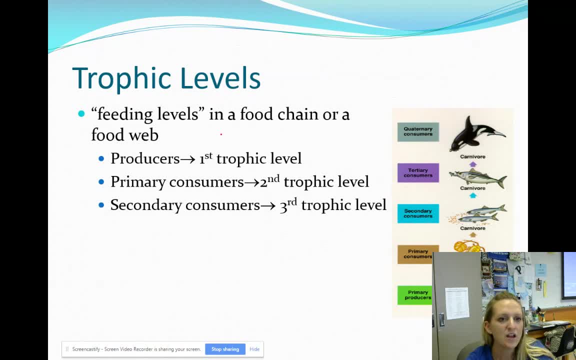 level in a food chain or a food web. uh, we're always starting with the producers. That's your first trophic level. Then we go to the first consumer, the first eater, the first one that takes something in. It's your second trophic level. Your third trophic level is going to. 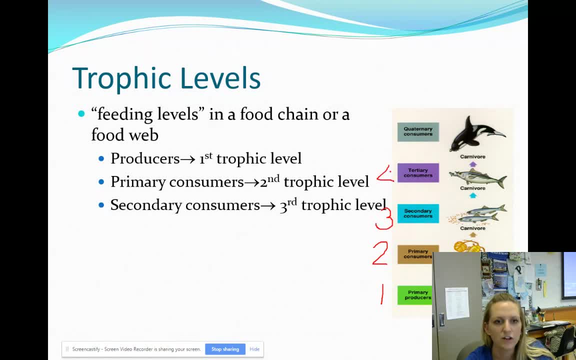 be a secondary consumer. The second eater, your fourth trophic level are tertiary consumers and your fifth trophic level is a quaternary consumer. We don't really go any higher than that because, remember, every step you go up you only get 10% of the organism below you. 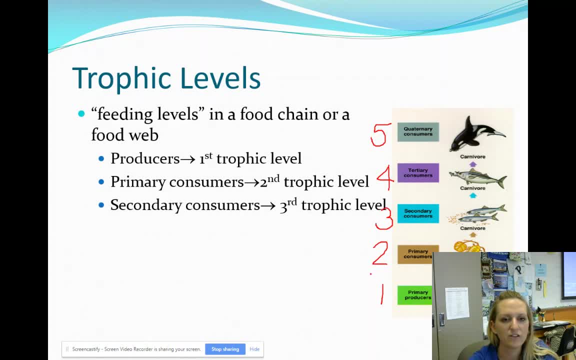 10% of the energy they had. Where does that other 90 go? Well, for example, phytoplankton is going to use a lot of it to do its phytoplankton thing: to reproduce, to photosynthesize, to move. 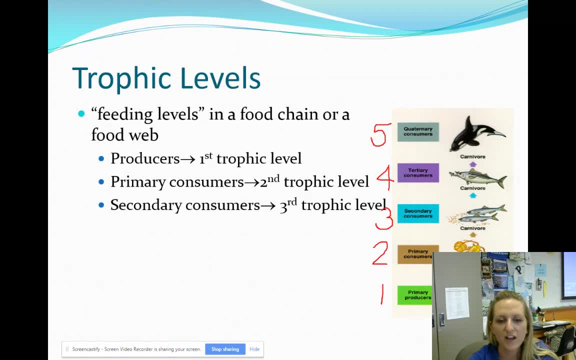 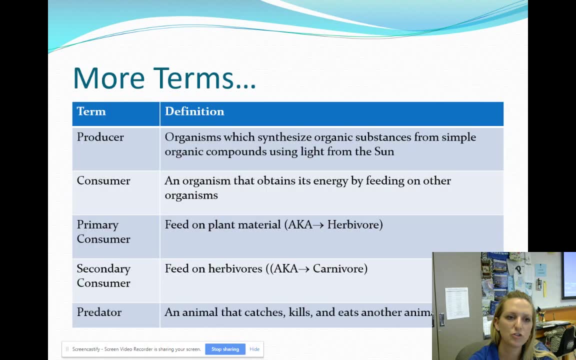 to um fight off any kind of infection, And then we have some of it that also goes as heat to the um environment, Trophic levels. Okay, A little bit more definitions. A producer is an organism that synthesizes organic substances. Don't say make, say synthesize, Don't say food. 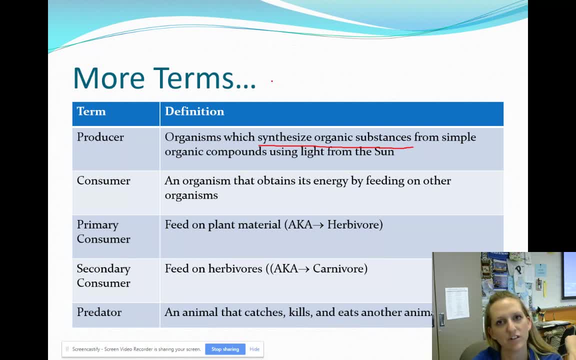 say organic substances or organic material, Stop saying food. They make food, Synthesize organic material. They synthesize carbohydrates from simple compounds using light and the sun, And those simple compounds were water and carbon dioxide. A consumer is an organism that has to get energy by feeding on something else, Even if it's a plant. 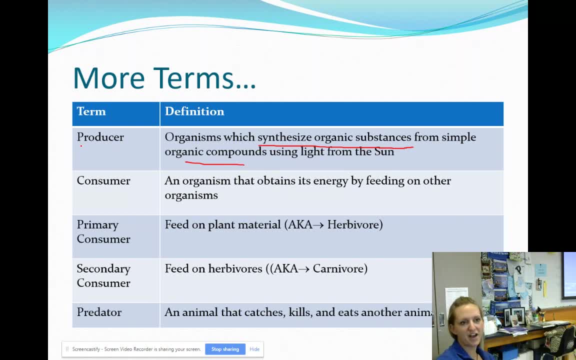 um, within your producers you have a photo- auto-troph and a chemo- auto-troph, auto-troph, auto Right, That means self, and autobiography is a book written about you by you. So auto is self, Okay. Um, and then trove auto-troph. We're going to go back to that trophic level. That means 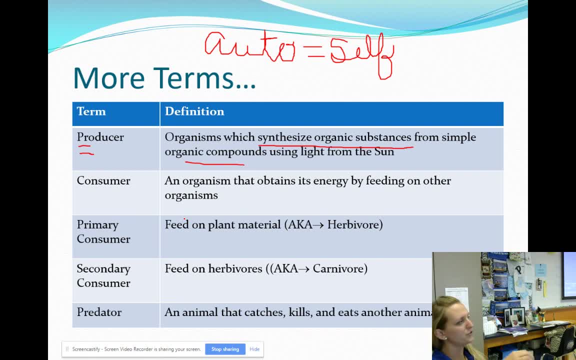 nutrient or feeder. You're a self feeder or self nutrients. You make your own photo auto-troph sun self feeder. You feed yourself with the sun chemo. auto-troph Chemo is chemical auto itself. Troph is feeder or nutrient. They make their own food with. 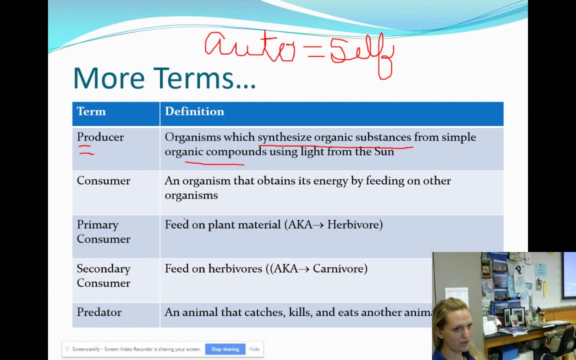 chemicals. That chemical is hydrogen sulfide, H2S, Um. primary consumers eat plant materials. You can call them an herbivore. Secondary consumers feed on the herbivores- You can call them carnivores. And then your predator is an animal that catches and kills and eats another animal. 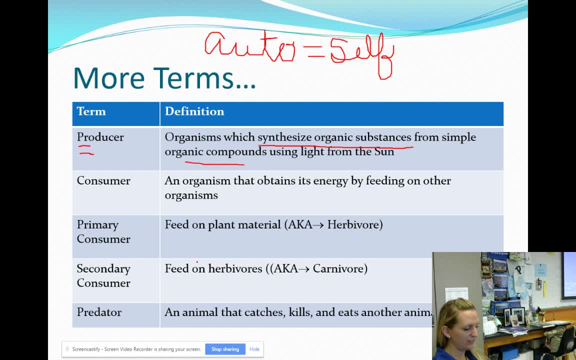 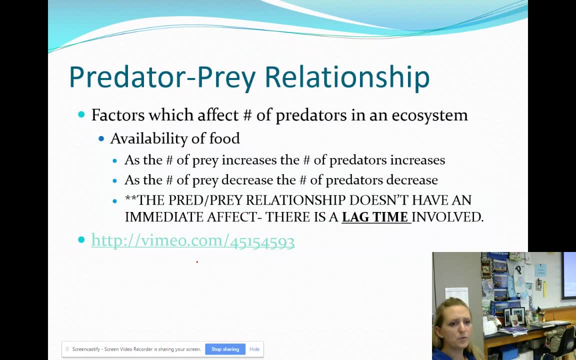 So a predator is not a parasite. A parasite is just like a predator. They're not stealing from you, They're not murdering you, They're eating you. They're just stealing. Predator- prey relationship. Um so we've also discussed this in all of your 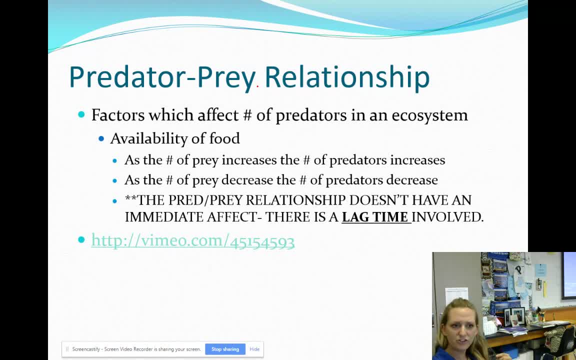 biology classes. This is a cyclical relationship. They control each other. Um, this depends on the availability of food, right Predators and prey. So as your prey population starts to increase, let's say, your, your small fish, your shark population can start to increase If your shark population gets too big. 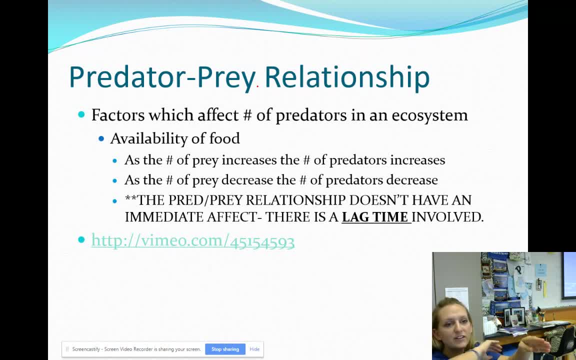 they're going to start to eat too many fish. Well, that sucks. The fish population is going to go down, and then the shark population is going to go down, And because the shark population continues to go down and there's less predators, Now the fish population can pop back up. 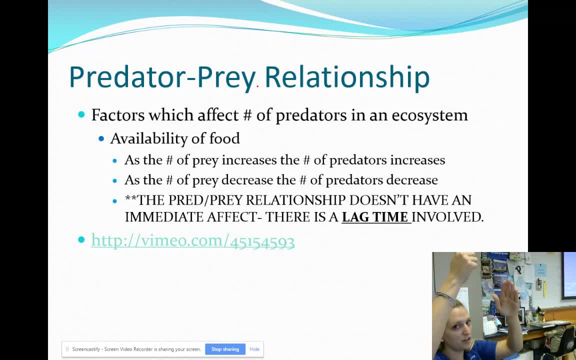 And as the fish start increasing, over time the sharks will start increasing, And then there's too many sharks that eat too many fish And then the fish go down. So then the sharks will start to starve and go down. They compete, sharks go down. 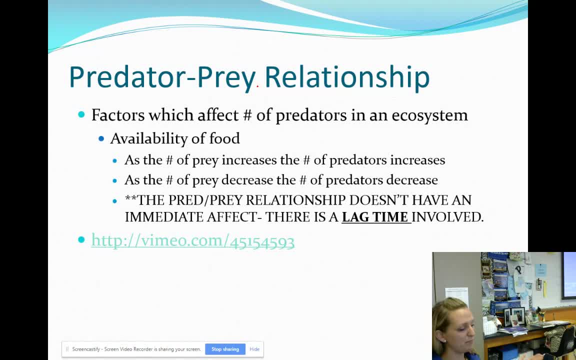 fish realize that they come back up and there is a lag time in between. It's really important for all these predator prey examples or looking at a predator prey graph. You always, always, always need to mention that there's a lag time, right A lag If your computer or internet is. 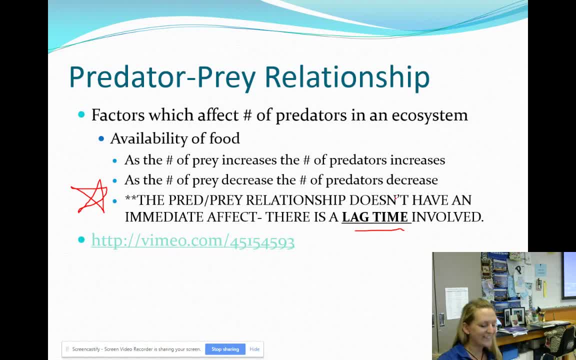 lagging, it's going slow, And this is because it's not like when sharks start to starve They can die. Fish are not watching them and saying: oh my gosh, that shark just died. We can have 20,000 more kids and immediately here come out 20,000.. It doesn't happen. It takes some. 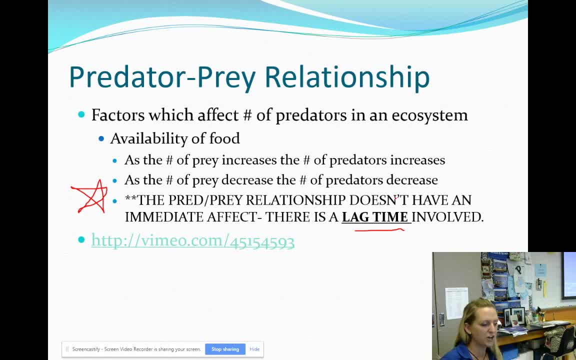 time for the environment to realize that there's a loss of predator and your prey, for example, in this one, your fish can start to mate, find a habitat you know, have their eggs, lay their eggs. Those fish grow, move on to a, you know, large enough size that they're going to be eaten. 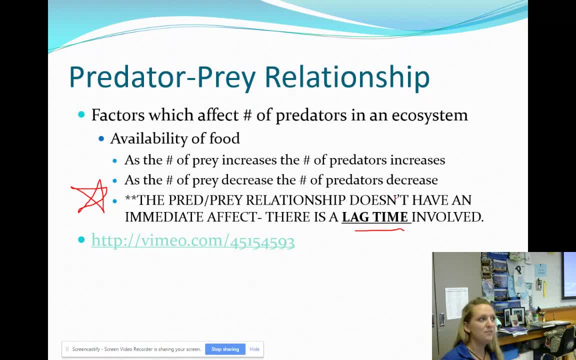 It takes some time. Likewise, as your fish start reproducing more and they're starting to grow, it's not like the sharks are like: oh my gosh, they just laid 20,000 eggs. Quick, here's 20 more sharks. That doesn't happen. It takes time. We have to be mentioning the lag time. 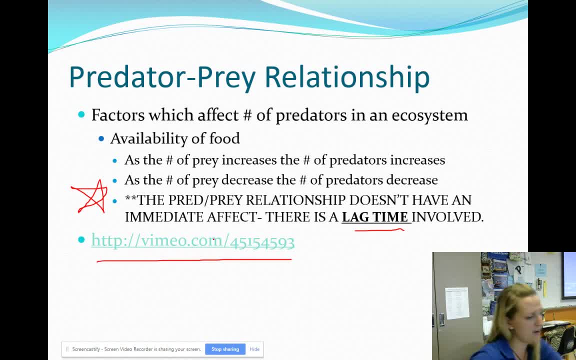 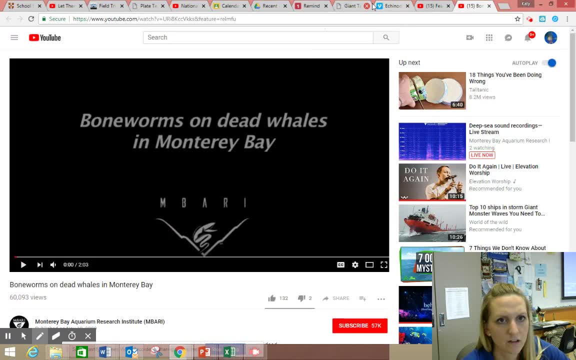 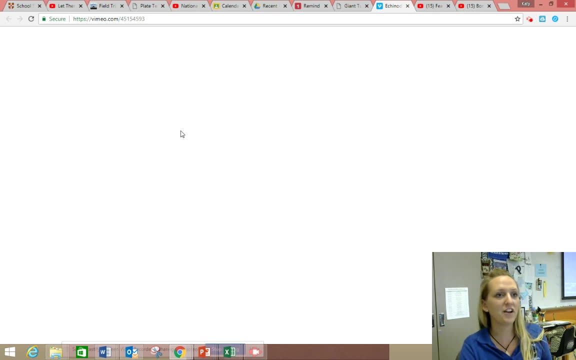 This is a cool video. Watch it, It is. this video is: um, uh, sea stars feeding on mussels And a lot of you guys, um, it's just going to take too long to actually show it. Please watch it. Um, a lot of you guys have, or people have asked me before. 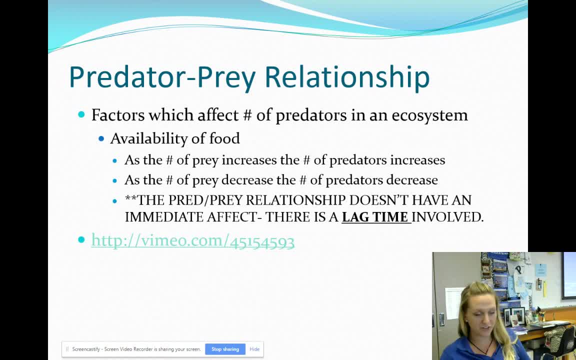 um, how do starfish eat? And it's they, you know. eject out their stomach into their prey. They ins. there's a tiny, tiny, tiny, microscopic video camera inside of the muscle And you can see in real time. it is sped up. You can see this happening. There's stomach coming into the muscle. 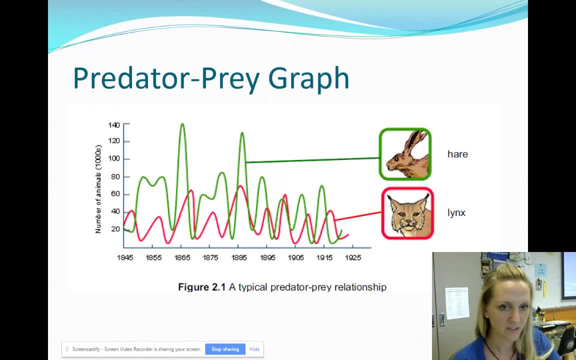 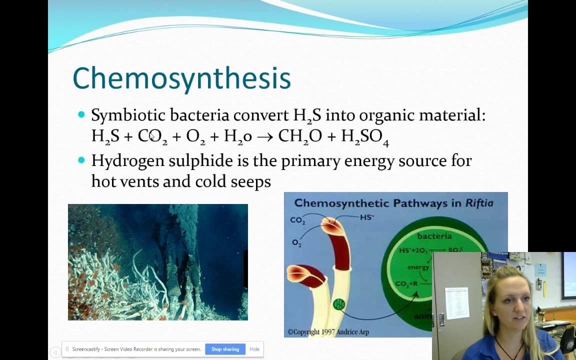 And then dissolving them. Watch it, Okay. Typical predator prey relationship. There is a lag time. Nothing is happening simultaneously. Okay, Chemosynthesis. Back to my pen. All right, So here's your hydrogen sulfide. They also take in carbon dioxide. 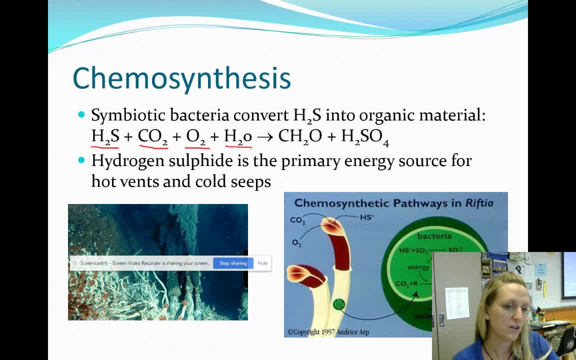 They also take in oxygen because they need to do cellular respiration. They also take in water. They can create their sugar. Remember it's a carbohydrate. Carbohydrates are carbon hydrogen and oxygen and a one to two to one ratio. Glucose is C6H12O6.. One to two. 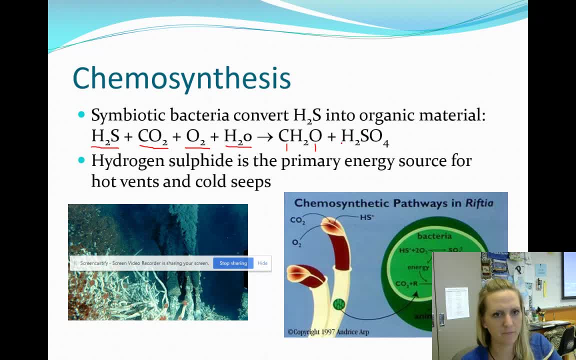 to one, And then they can also produce- um, this isn't sulfuric acid, You'll remember. I would say hydrogen sulfate, because I know SO4 is sulfate. I don't know, You guys took chemistry last year. So hydrogen sulfide is the primary energy source for hot vents and 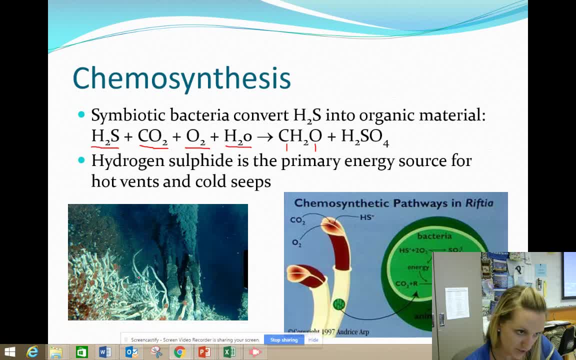 cold seeps, which are your hydrothermal vents. There they are, Black smokers, All of your tube worms. There's so many, Okay, And down here is where your chemosynthetic bacteria live. They're doing chemosynthesis inside of the tube worm. 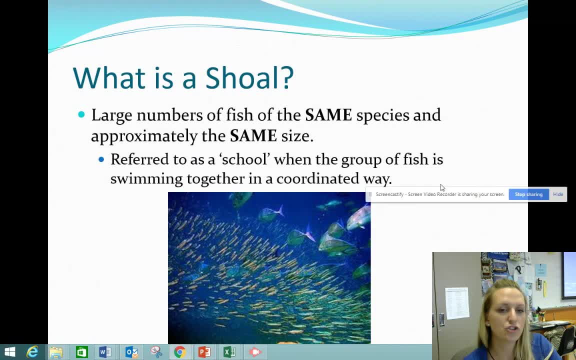 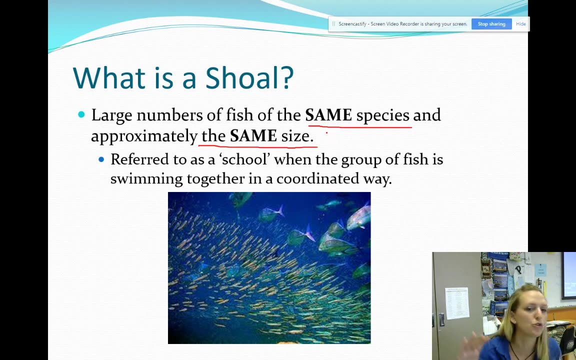 Riftia, What is a shoal? A shoal is like a school, but it's not called school. So it's a large number of fish of the same species and approximately the same size. This should make sense. You can have adult grouper shoaling together. There is not going to be juvenile. 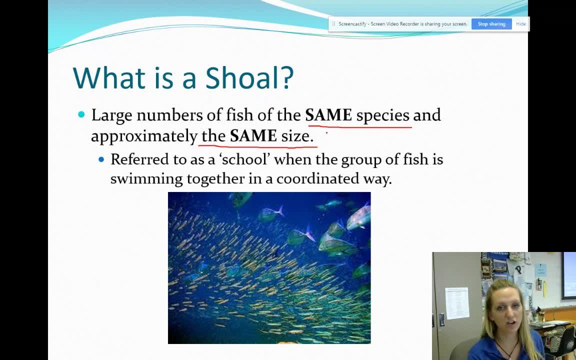 grouper there, The juveniles are going to be living somewhere else. When we talk about a level and we talk about, um uh, marine reproduction and fish reproduction, they're you know. it's like their families. the. the different age groups are so split apart from. 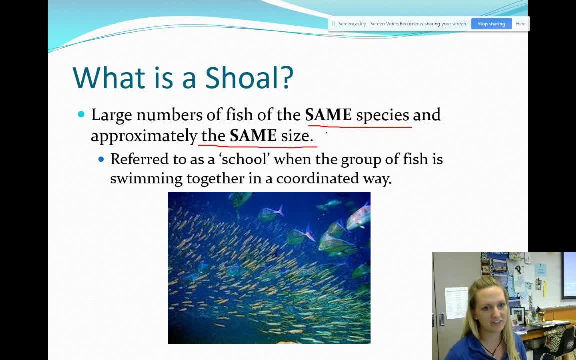 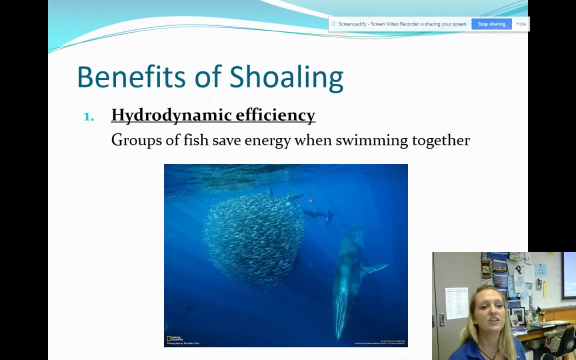 each other. So a shoal is same species and same size. same species and same size shoaling together can be referred to as a school, when they um group of fish are swimming in a coordinated way but they shoal. Why? What are the benefits? You guys write all of these down Many times. 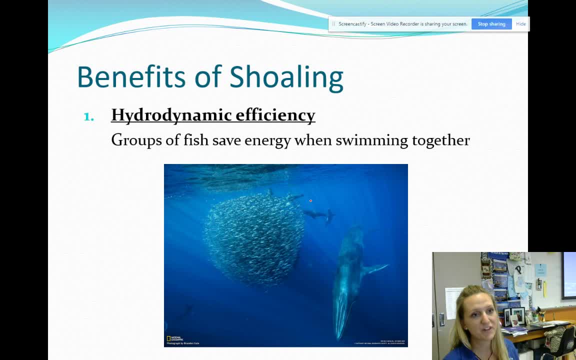 this question is like an eight point question And it's not hard. So what is the benefit of shoaling? Um, if there is a hydrodynamic efficiency? so you know if you are more aerodynamic when you're just swimming in a group. they're like 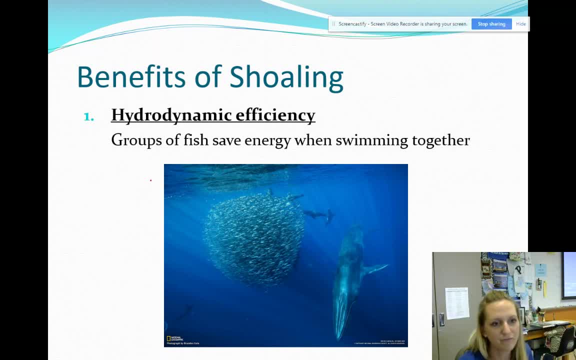 following the current of each other. So if you have, you know, 4,000, 5,000 fish also being in the same direction, you might not even have to swim too hard. You're just going to follow it because that's the way the current's going. So it's, it has a hydrodynamic efficiency. 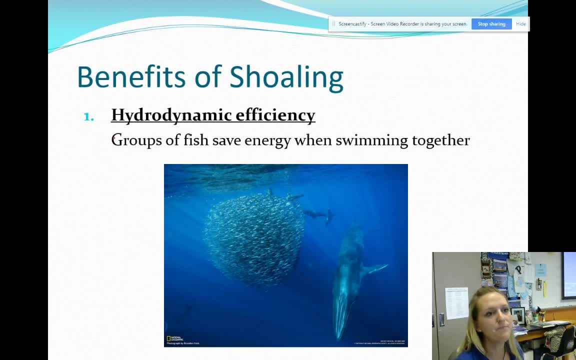 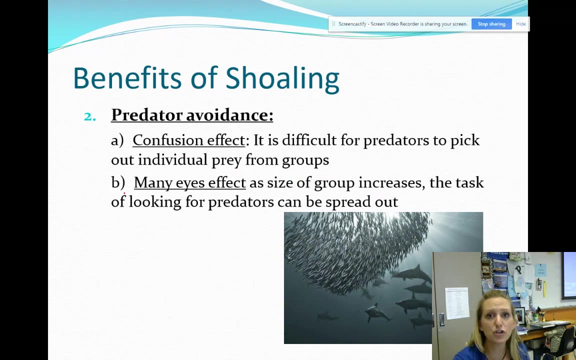 And list the benefits of shoaling. This could be an acceptable result right here. One of them Now, if it says: explain the benefits of shoaling, you need to give this and this and the Y: predator avoidance. Okay, For there's two ways that they can avoid predators: by just being. 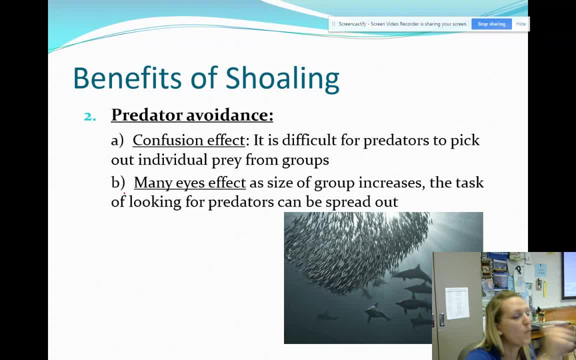 confusing. Um, it's difficult for predators to pick out one fish when you have a a shoal of thousands of fish. Also, they can avoid predators by, like you know, safety numbers, the buddy system, all of these different eyes looking. 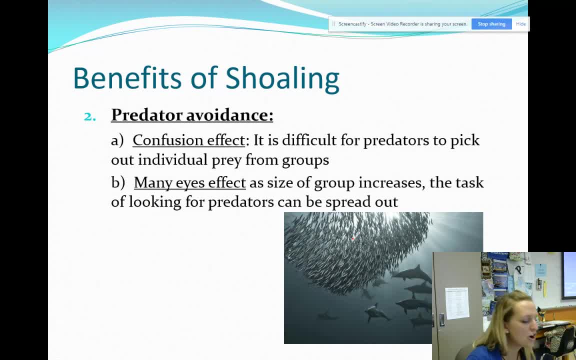 at all different directions. They're looking out for predators. Fish are amazing. They have on the side of their body- it's called a lateral line, and they can sense any sort of movement. You have all experienced this, I'm sure, if you've ever been near water. 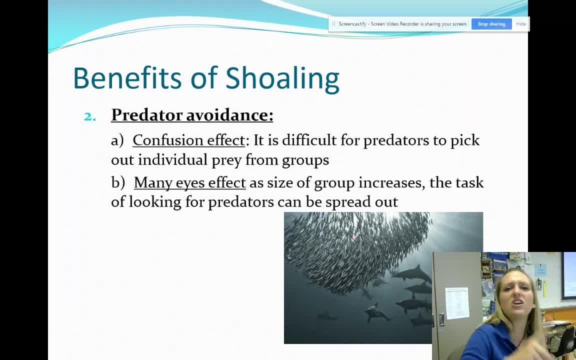 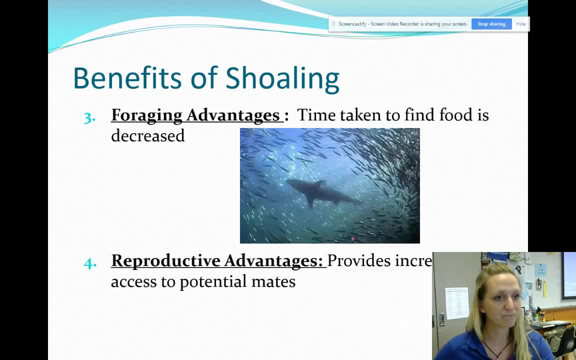 um, you know, you're, I'm going to grab that fish. I'm going to grab that fish And you can't even like, touch the top of the water and that fish is gone. They all are really great at coordinating something together because of that lateral line. Okay, There's foraging advantages. You. 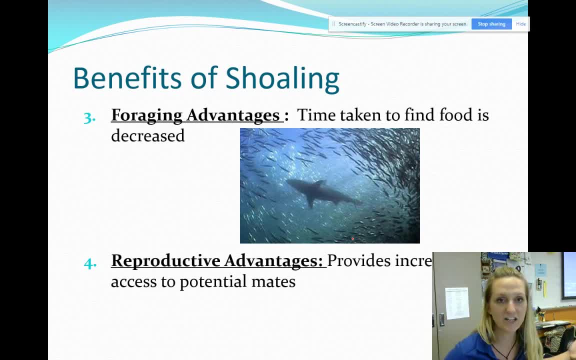 you know, if there's 5,000 of you hunting for food, it's not going to take too long. The time taken to find food is decreased. Okay, This, this isn't discussing this, but that can also be a disadvantage, because it could cause competition. Um, there are reproductive. 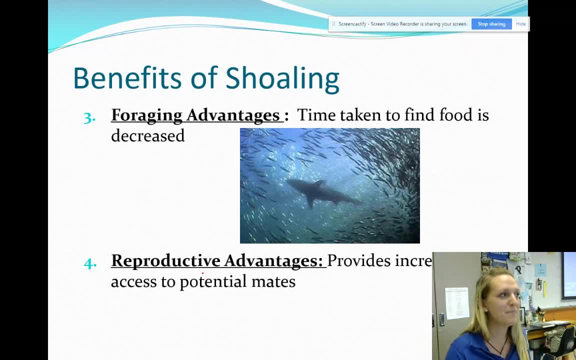 advantages. You know, you don't have to find a mate If there's 5,000 for you to find, it's way easier Searching around for it. So having a group of five, 10,000 fish together, you can find a mate way better than if it was, you know, 20.. 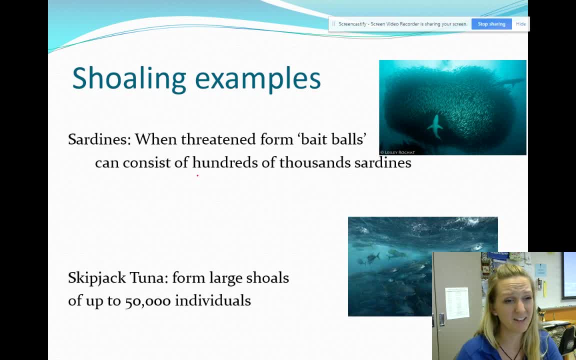 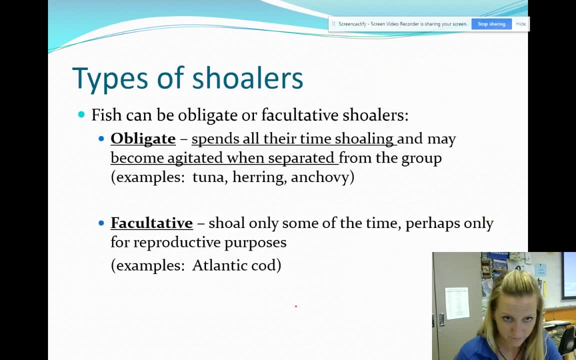 Okay. So an example of sardines. they form bait balls can meet hundreds of thousands of sardines. Skipjack tuna can form shoals of up to 50,000 individuals. Types of Schollers: Um, this is covered in the text. It really hasn't been covered heavily on. 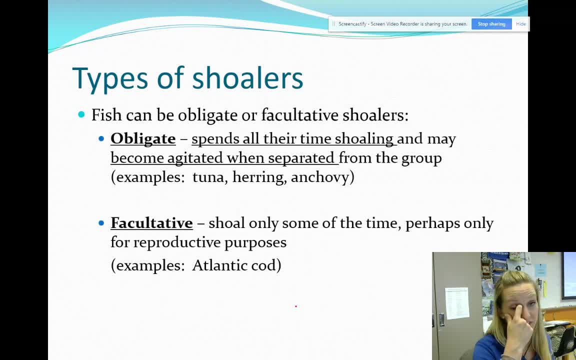 any papers. So I would focus most on knowing what the benefits are and that saying: don't write this, write this, because if you don't write it, you know for sure it's going to be on paper one. It's just the way that's going to go. But there's two types of show shoulders. 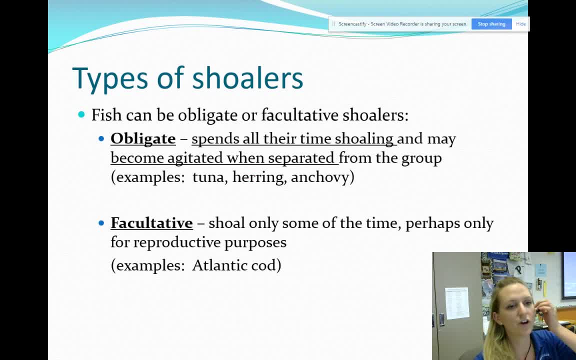 You could be obligate like you're obligated, So you spend all your time showing And when you're away from your group they get really agitated. They need to be in the group. Tuna, herring, anchovy, They're like that. 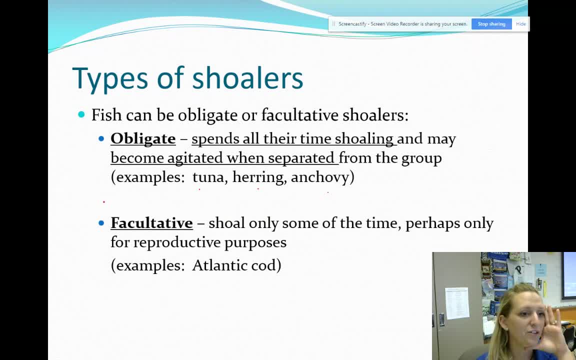 Or facultative, Facultative, I knew it, Oh my God, I'm a poor, I'm a poor one. Facultative, So they show only for a purpose, Like so, for a function, maybe only for reproduction or only to find food. 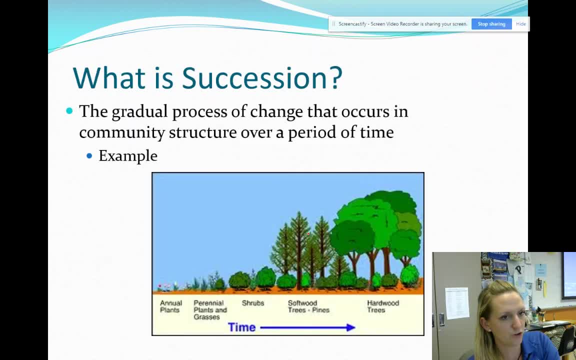 They're only showing that, not for like their life, just for a certain purpose- Succession. This was the quiz question today And you'll see the answers at the end of this. So you guys have seen this, a picture like this, when in your biology classes. 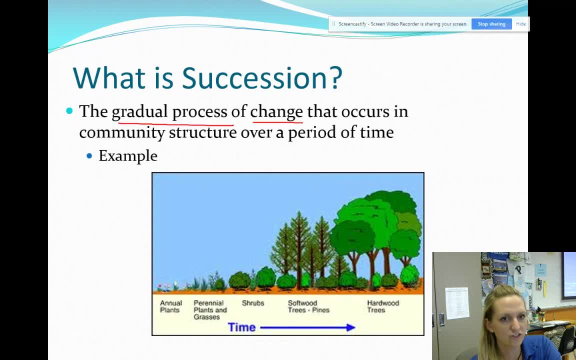 Succession is going to be a gradual process of change that occurs in a community over a period of time. Two point question, when you describe what succession is and then you're going to give an example, Yes, that would make it three: A gradual process of change in a environment or a community. 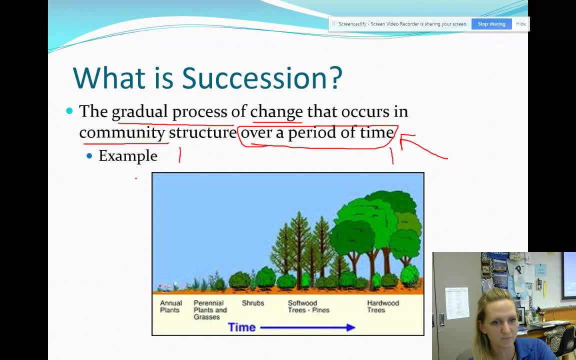 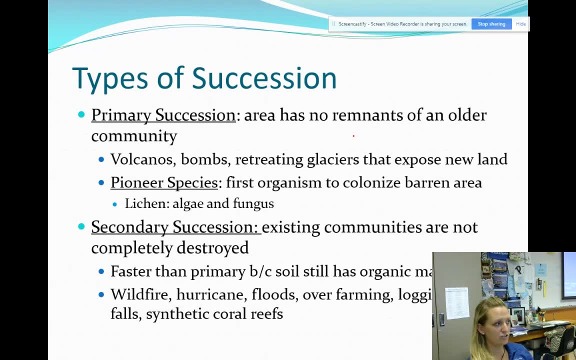 That's one point. over time is the other Point. Primary succession is worst case scenario. in primary succession, This would be like a bomb, a volcano, retreating glaciers that just scrape down all living material, that are on any substrate, you know whether it's rock or it's sand, and they're exposing new land, new land that has nothing living on it, nothing at all. 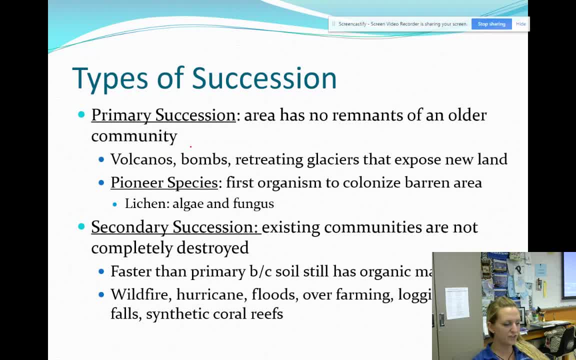 So primary succession: there is no remnants of the Older community that's living there, Nothing at all. There is no producer, There is nothing. The soil is not fertile. You got to start again from square one, Sorry. Secondary succession is a little bit better. 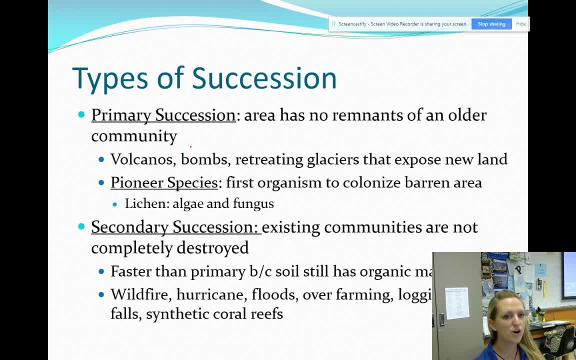 So secondary succession, we're still screwing it up, but your existing communities are not completely destroyed. So it's easier to pick back up your environment from a secondary succession versus a primary, Because primary you're starting with a blank slate. This is faster Again if we're talking about on land. your soil still has some organic material. 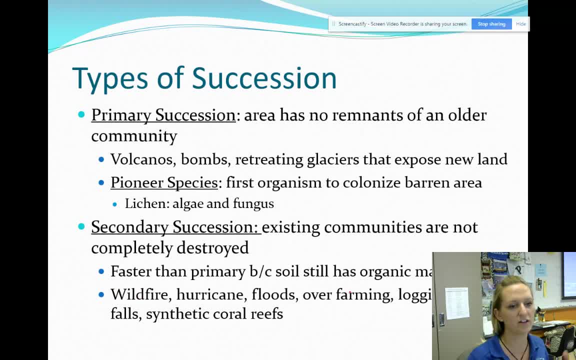 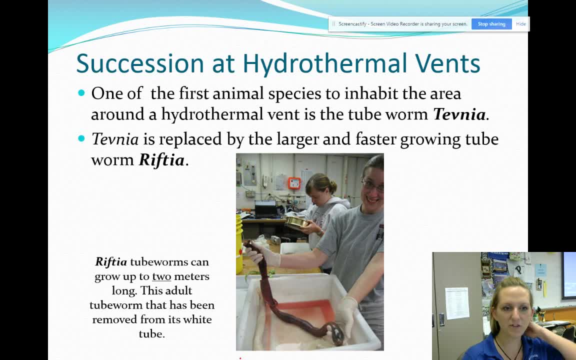 This would happen after a wildfire, hurricanes, floods over farming, lodging whale, fall, synthetic coral reefs, Succession at hydrothermal vents. This could have been one of your answers on your quiz today. So this is one of the first species that are going to inhabit a hydrothermal vent area. 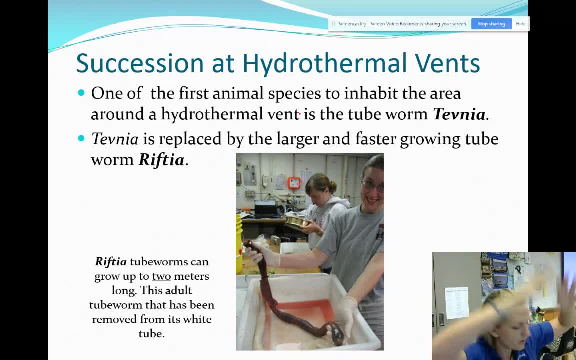 What So? like right when, Right when the mantle of the earth is coming out of the coming out of the ocean, the bottom of the ocean. Right, We have this underwater volcano happening. It's going to solidify and start to build your hydrothermal vents. 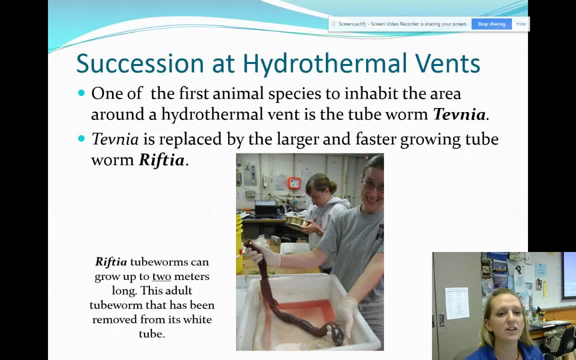 But right, when that happens, we have nothing living there in the first organisms- We call them pioneer species that are going to inhabit. There is this tube worm called Tevnia. Tevnia is your first tubeworm species, Right, She's to inhabit it after Tevnia kind of sets up shop there. 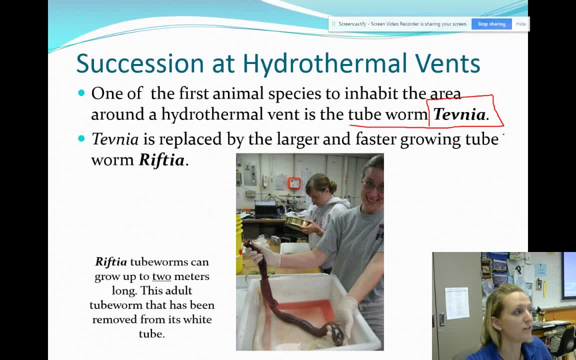 Tevnia gets taken over by a better, stronger, better looking to worm called Riftia. It's faster growing. Riftia can be up to two meters long. This adult, two worms and taken from its white to gross, It's just grossed. 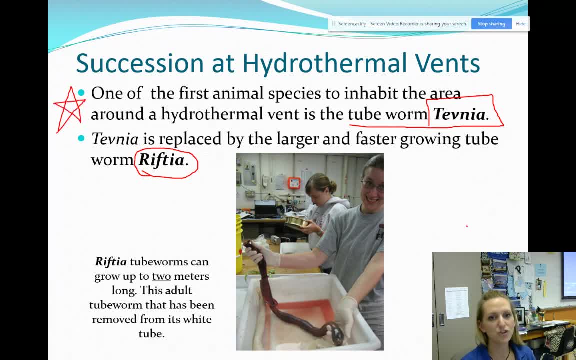 All right, Know this, You need to know succession. at a hydrothermal vent. It goes from Tevnia to Riftia. You're like what? What are those words? I know Literally. I know I taught myself this last year. 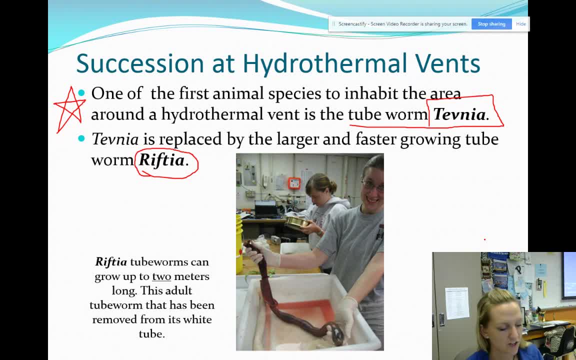 Tevnia and Riftia. I did not study hydrothermal vents in college, So you know, write it multiple times, Say it multiple times. You have to know it. Tevnia, And then it goes to Riftia, T and then R. Tevnia is little. 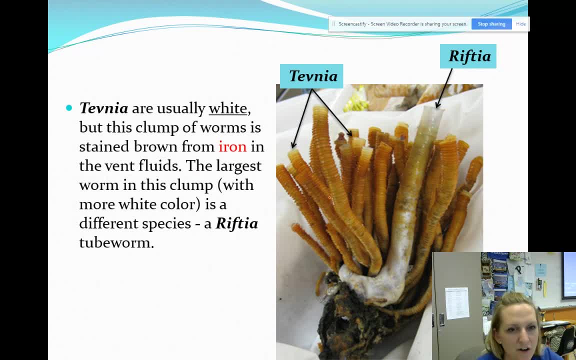 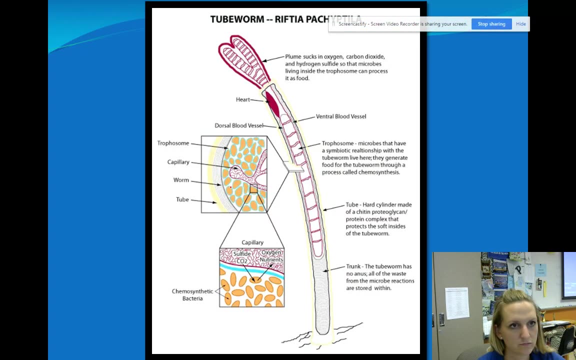 So they're usually white And it's stained brown here from iron, from the vent fluids, from like, because there's a lot of minerals coming out. Riftia is this longer tube worm, has that white titan shell? Okay, Again, Riftia. 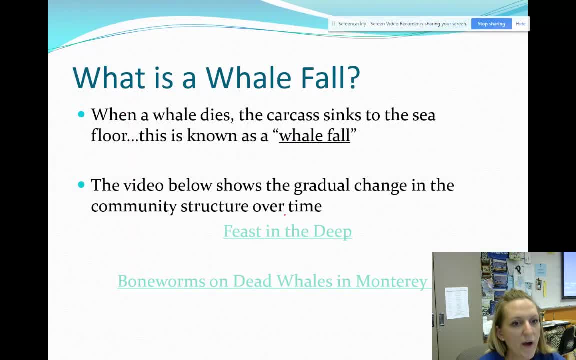 You don't need to know its body plan. A whale fall. Please watch both of these. They're awesome. They are awesome. So a whale falls also a secondary succession. This is when the whale carcass sinks and a new ecosystem starts to grow on it. 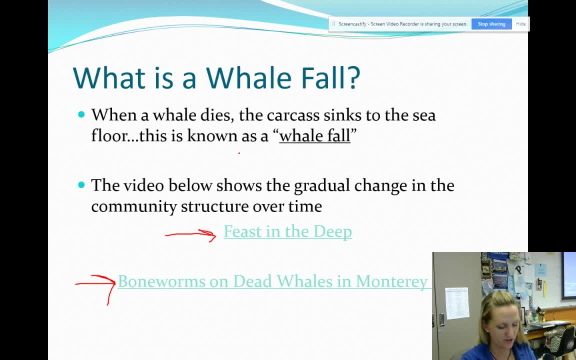 It's awesome, It's called a whale fall. This is another thing you could have written for your extra credit on your quiz today. Anybody who's maybe was absent on Friday and is taking the quiz on Monday, you do not get the opportunity for extra credit on the quiz. 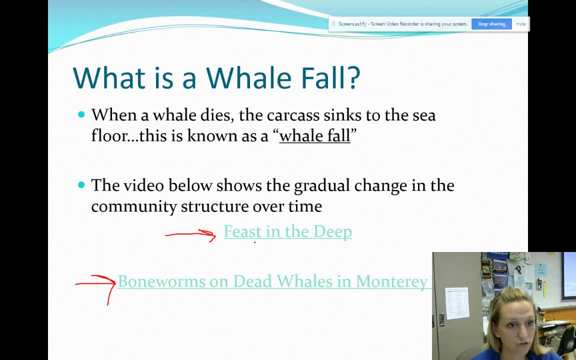 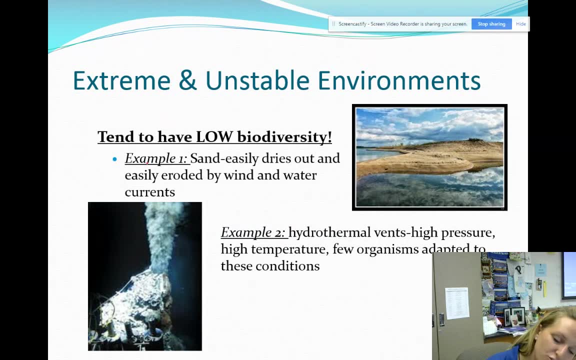 You have to be in attendance to have it. Okay, Check out these videos. They're awesome, We're almost done So. extreme and instability in environments. So, if we're looking, okay, extreme and unstable environments. So, talking about their biodiversity, they tend to have low biodiversity. 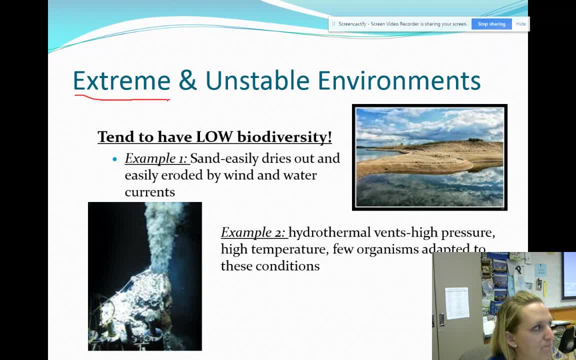 An extreme environment is going to be like the Arctic, like a glacier environment. It's going to be definitely your hydrothermal vent environment. That's extreme. You have really acidic conditions, So you have low pH where that's. that's acidic. 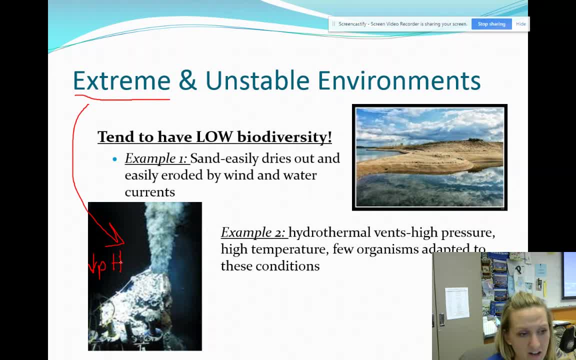 The pressure is unbelievably high. You have it's very dark, It's very cold, but right here at your vents the water is boiling, It is in and it's it's toxic. So that is going to have really low biodiversity. 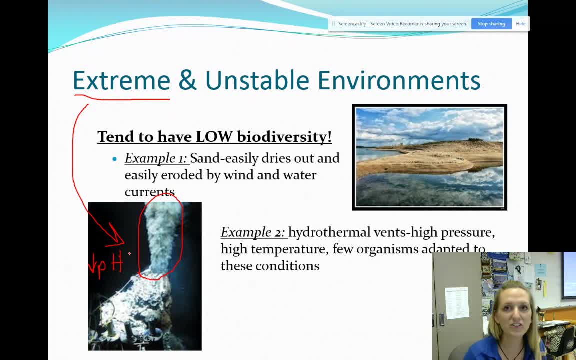 It is an extreme environment. It is a low biodiversity because not many organisms are adapted to living there. You need to have very specific adaptations to live there. Now, if we look over here um at a Sandy beach environment, this is also going to have low biodiversity. 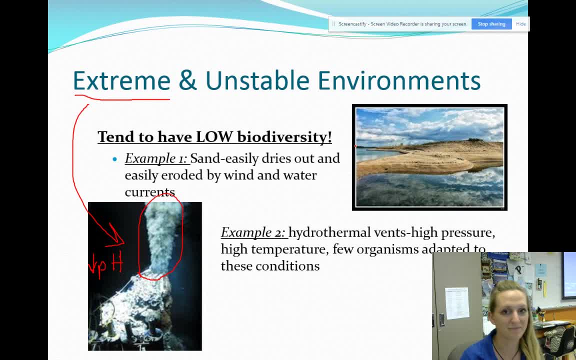 No, it's not extreme. It is not extreme, right, There's not extreme temperatures and the water boils and lightning strikes at this. It's not extreme. The pressure isn't too high, The temperature isn't horrible, Okay, Okay. 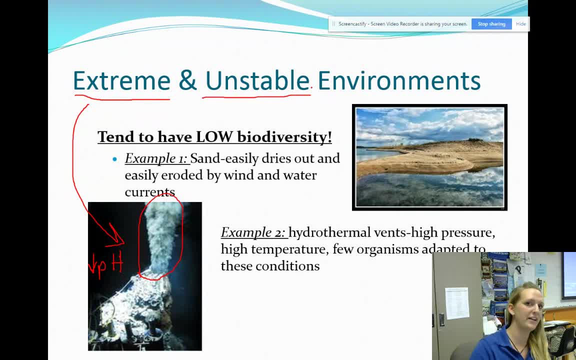 But it is unstable because you have the tide coming in and out. Um, you know it? ha, it's really susceptible to weather patterns and weathering. You can have organisms drying out easily, So for that you have to have certain adaptations to live there. 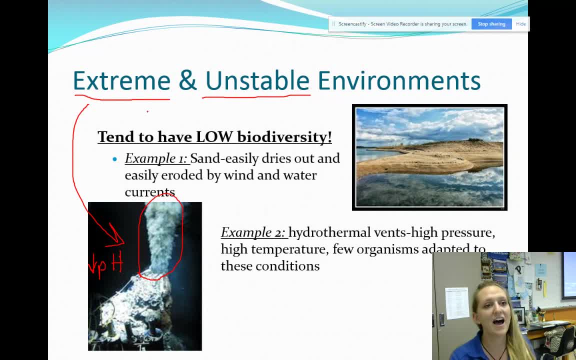 It is not a stable environment. It's not extreme- This one not extreme, but it's not stable. Doesn't stay the same. Hydrothermal vent: It is stable. It does not change that often. Nothing's changing it. The tides going in and out is not changing it. 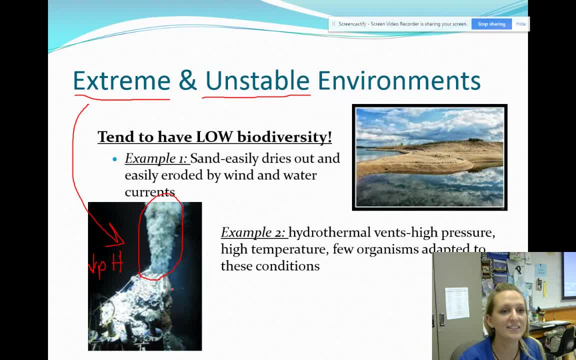 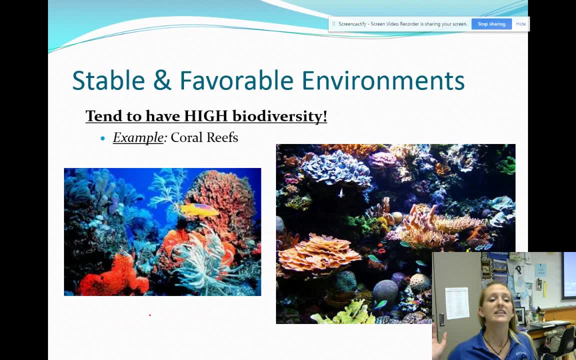 The sun rising and setting is not changing it. It's stable but it is very extreme. The conditions are extreme and they have low biodiversity. Now, if you have a stable and favorable environment, you're going to have very high biodiversity. So the temperature, you know, stays a relative constant or maybe only fluctuates within 20 degrees. 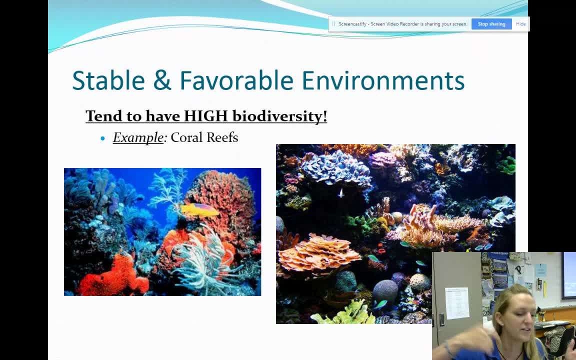 Um, the pressure Pressure isn't too high, So you're not too far in the depths. The salinity isn't too high. The pH isn't crazy. Um, you're not exposed to sunlight. in in almost drying out, It's stable. 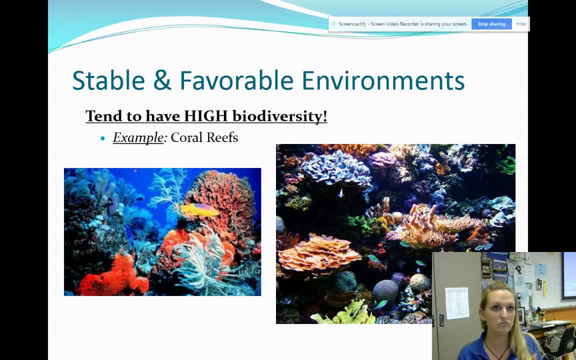 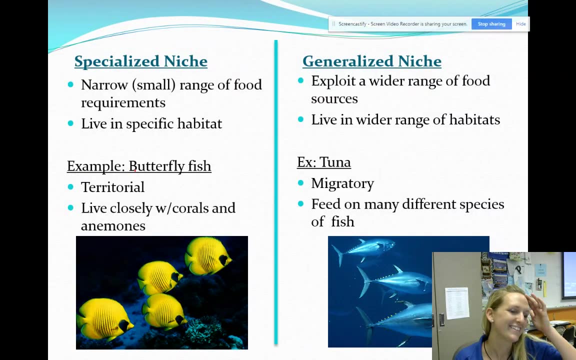 Coral reefs. their environment stays stable all the time almost, And it's favorable. It is not extreme, So you're going to have high biodiversity. There are a lot of organisms can live there and tolerate it. Two more sides Okay. 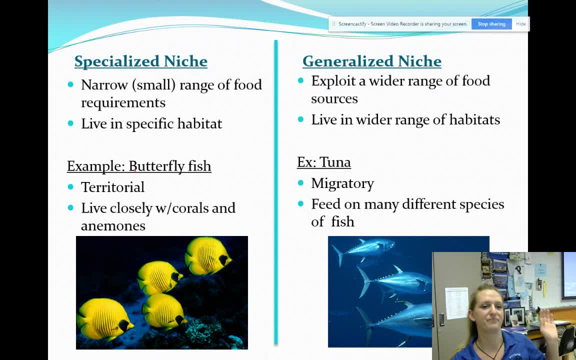 A specialized niche. areas that have high biodiversity, high bio diversity, are going to have very uh. well, we're going to say they're specialized niches. Why? All right, Think about, think about it- Coral reef. There are so many species, different species, that live there. 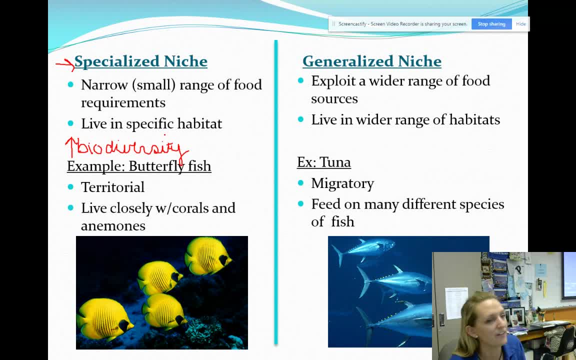 They can't all be doing the same thing, eating the same thing, living in the same place, or there's going to be problems. So we say they have a specialized role. Um, we also say they follow very narrow food requirements. There are so many organisms that we can't in the coral reef. 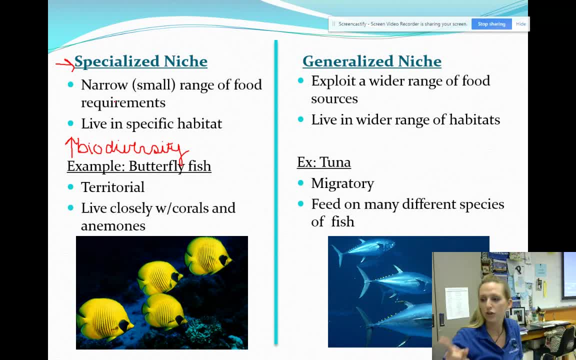 We can't say, okay, you guys can eat all of this. No, You Can have this, you can have that, You can have this, you can have this, you can have this. you can only live right here and you can only live right here, and you can only live right here. 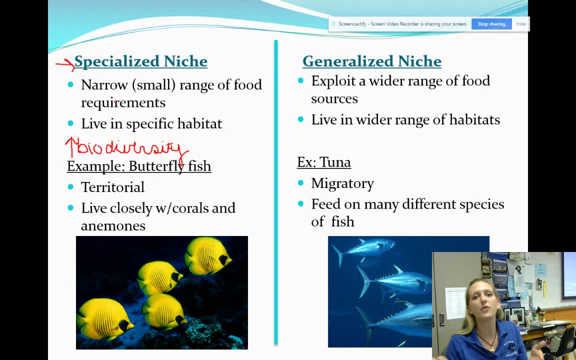 And so we have very narrow ranges of where they can live. Otherwise it's going to cause overlap. If two different species are sharing a food source competition, two different species are sharing a habitat competition. So we say they um places with high biodiversity or coral reefs are going to have very specialized. 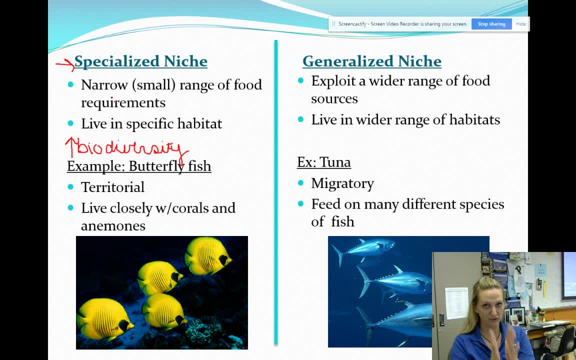 Misha's, because they can only have a narrow, you know small area of where they can live and what they can eat. specific habitats- There's just so many there They they have to have like a purpose and not overlap Somebody else's. butterfly fish is an example, because they live in coral reefs. 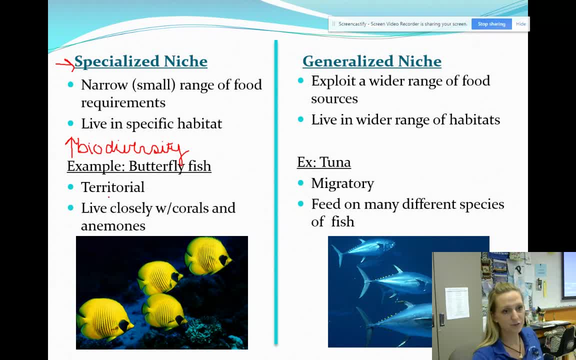 Any organism that was in coral reef could be an example. Um, these guys are territorial, They live really closely with corals and an enemies generalized niches. So, um, it's general. you know these. these are organisms that can live in a wide range of habitats. 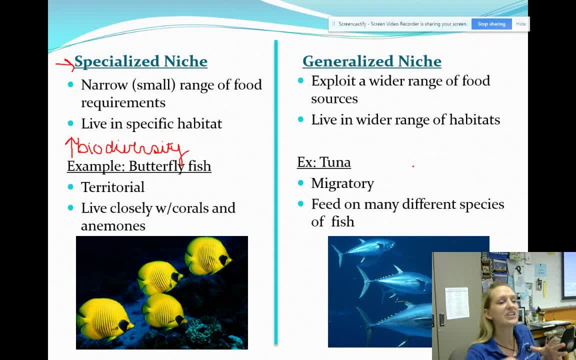 Um, therefore, they are not stuck to just eating one type of food source all the time. No way, they are migratory, They can. you know, like sharks, they can live in multiple different kinds of salinities, temperatures, pHs, where, like our corals, Scott, to have a stable pH, got to have a stable salinity, got to have a certain depth, got to have a certain temperature. 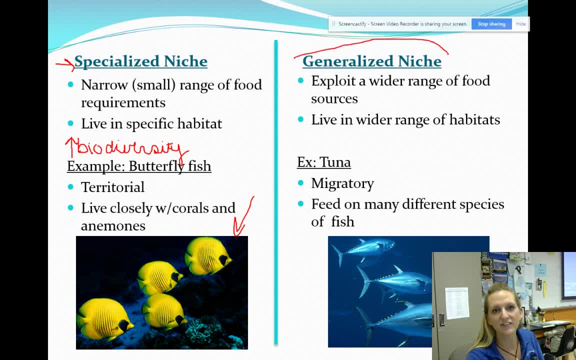 But these are going to be over here. Your generalized niche are going to be organisms that don't have to stay in a certain temperature, certain pressure, certain salinity. They can kind of move around- Um, a shark is a great example of this- so they can exploit a wide range of food source. 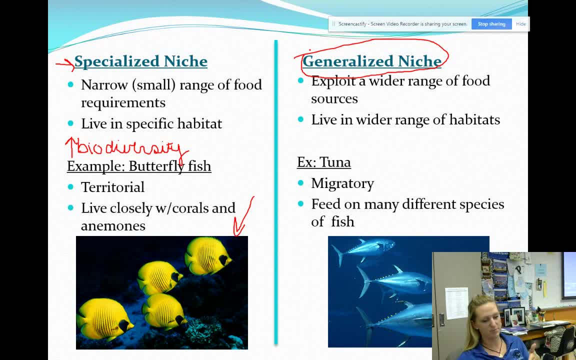 Again, our shark. they're not stuck to just eating one thing because there's so many of them. No, they can live in a big area, so they can eat whatever the heck they want. They can also exploit a wide range of habitats. 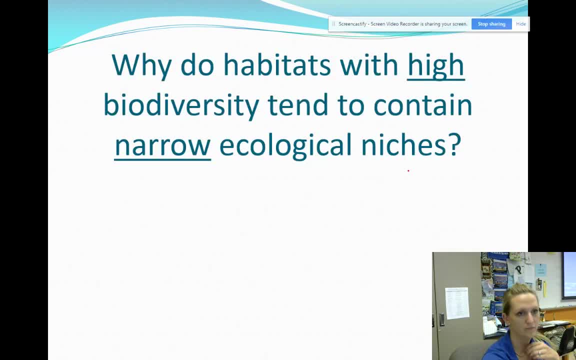 Sample is tuna or a shark. Okay, Okay, Very common question. Why do habitats- and, it would say, explain why habitats with high biodiversity- tend to contain narrow ecological niches? Each species has its own niche in the ecosystem. What would happen if the niches overlapped? 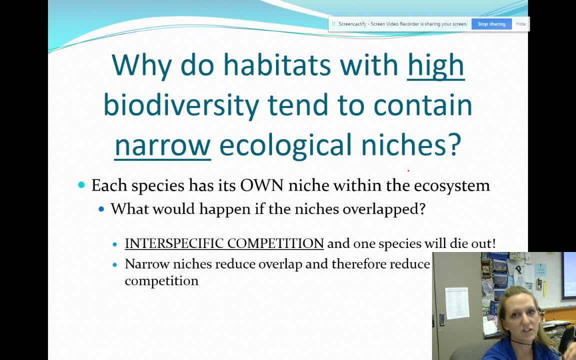 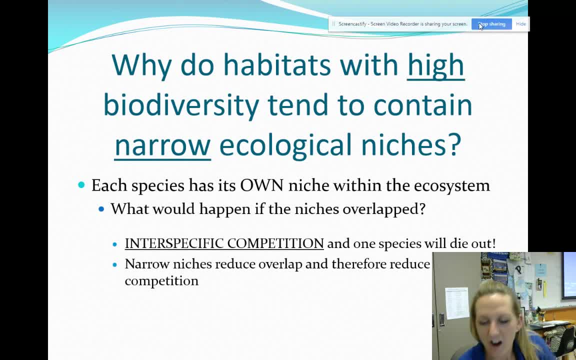 We did it, We did it, We did it. Good job, guys. All right, let's see your test over this, and now we will be practicing, practicing, practicing, practicing. Your chapter two test is um Thursday the 13th.